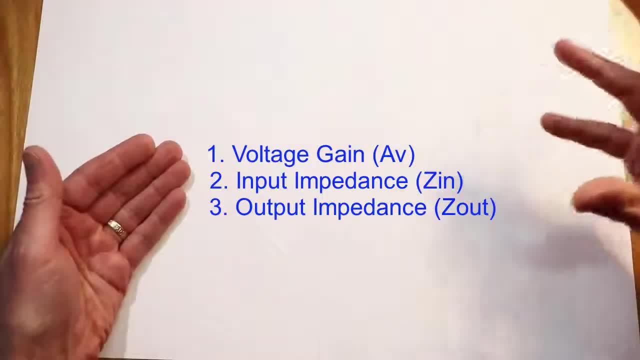 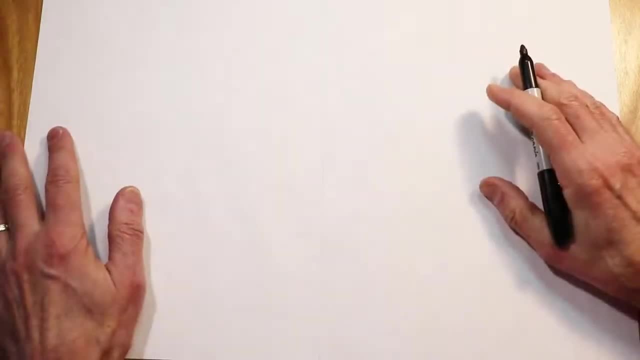 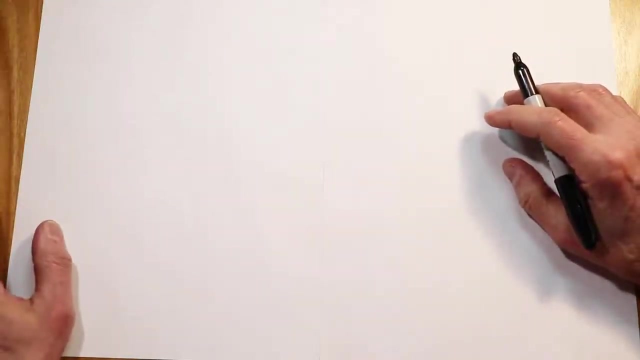 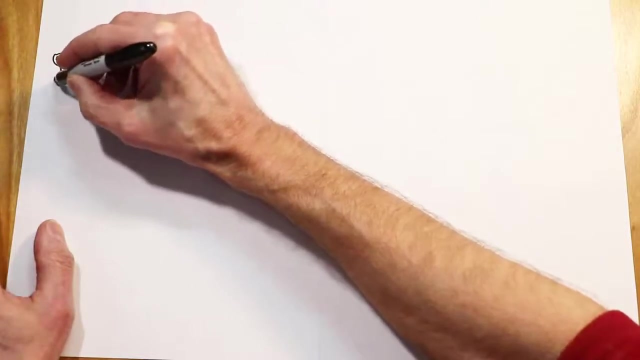 its output impedance. in other words, what does the load see as far as the impedance that drives it? Now, there are many ways that we can bias this particular circuit For no particular reason. I'm going to use a voltage divider bias- Very handy if we have a single power supply. So we will start with a nice AC source over here. So this will be our VN. 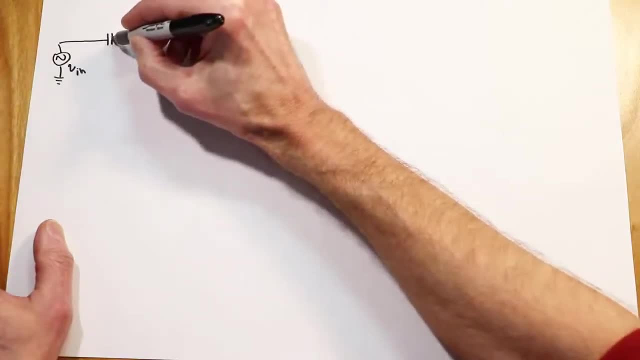 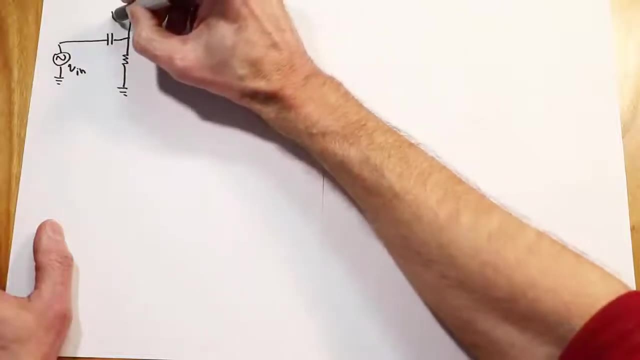 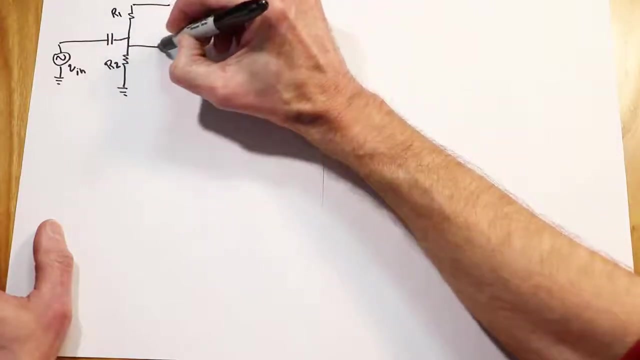 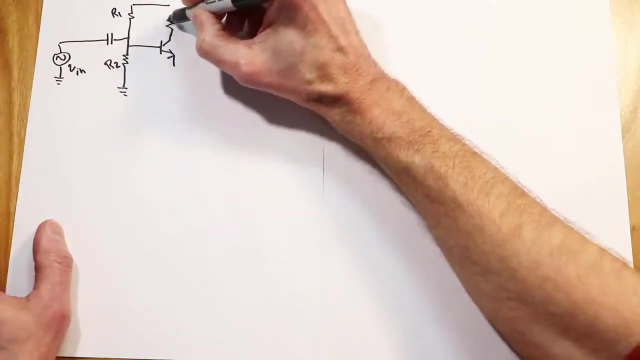 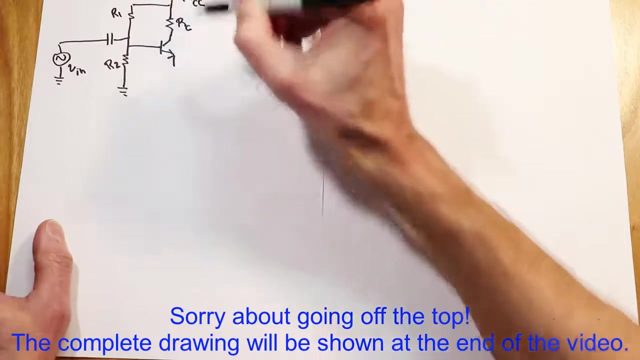 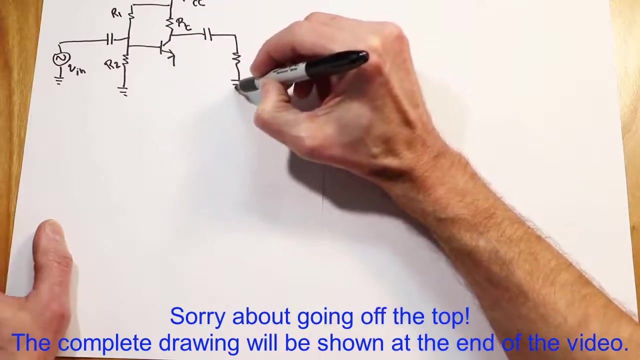 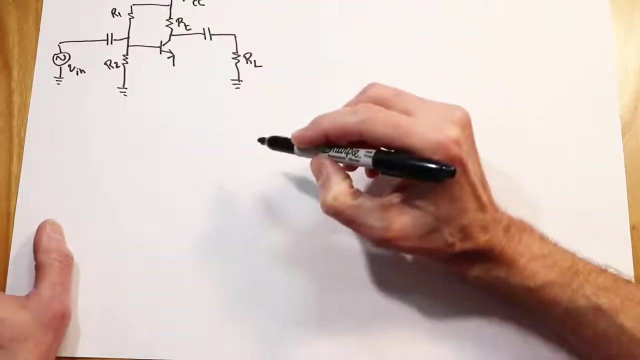 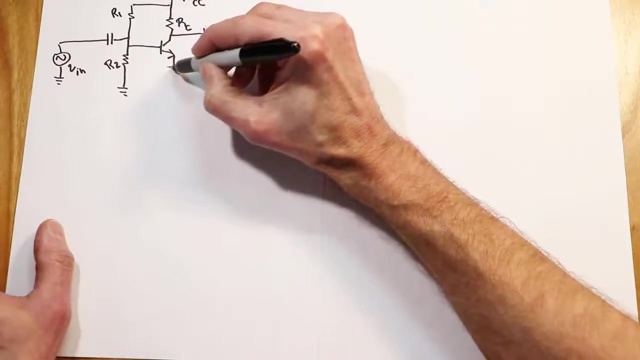 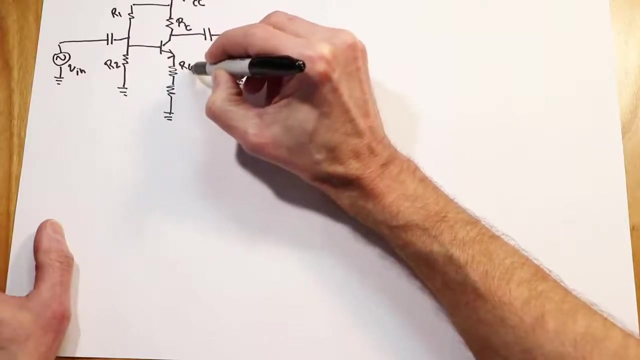 And this is going to come in through a coupling capacitor, through a couple of voltage divider resistors. We'll just call the one on top, R1, R2. on the bottom there's our transistor and we have a collector AC. Off of this we have a coupling capacitor which will go to our load, the thing that we are driving. And then I'm going to do something a little bit different down here in the emitter. Normally on a biasing circuit we would just have one resistor going to ground here, but I'm going to split that in two. I'm going to have two resistors here, And the top one I'm just going to call RE1. 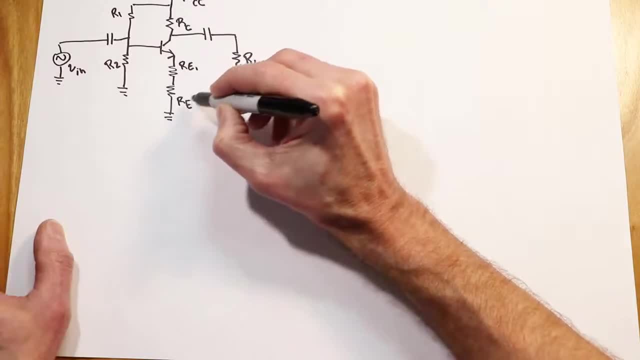 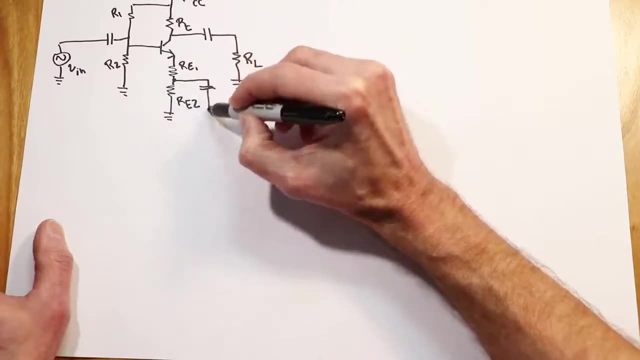 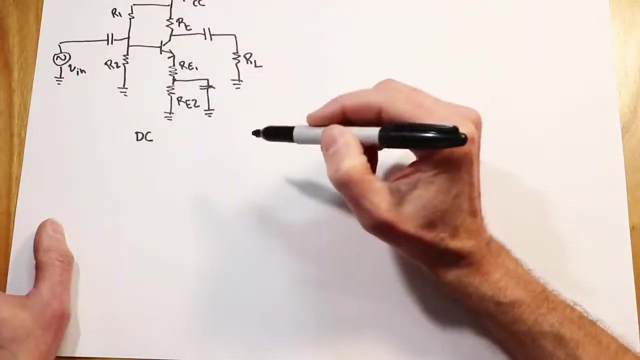 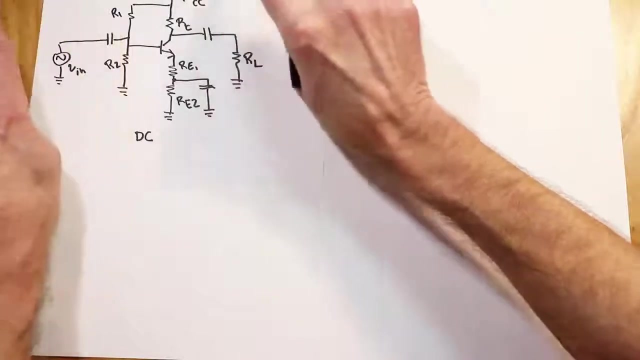 And the bottom one I'm going to call RE2.. How inventive. And in between these two we are going to place a capacitor, a bypass capacitor. Now for DC. these caps all open up. Basically, the AC source disappears, the load disappears because these things are open And then because this coupling cap opens up, essentially the DC emitter. 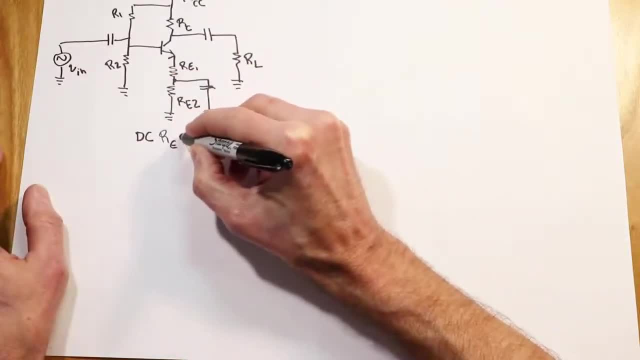 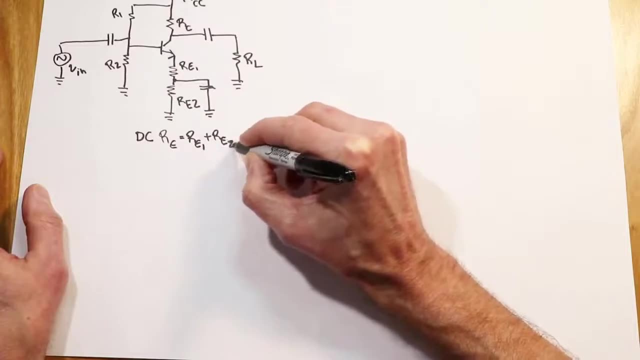 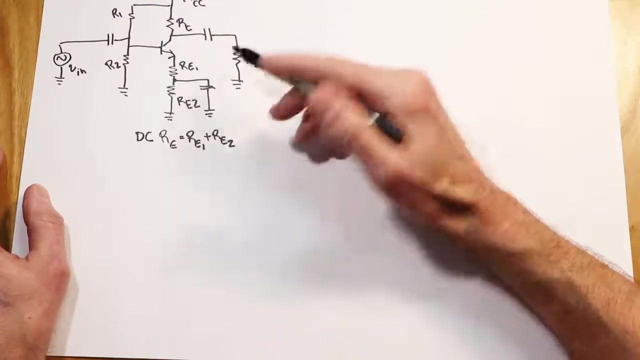 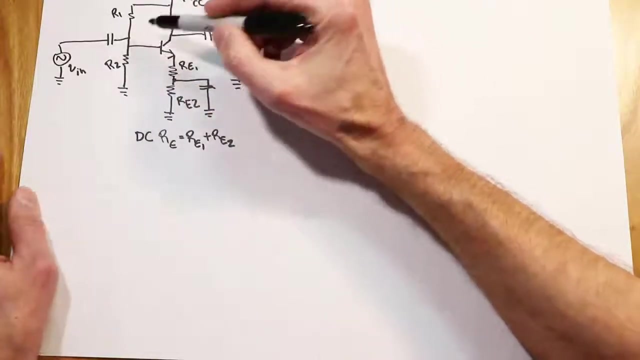 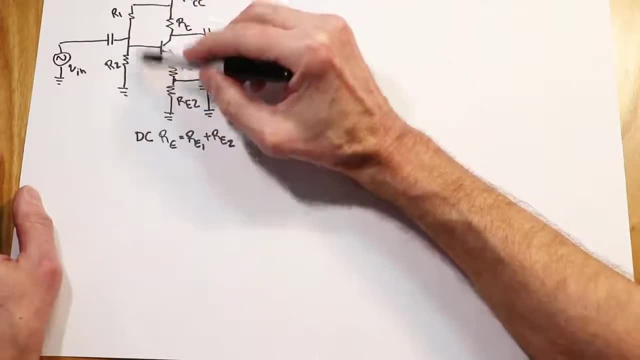 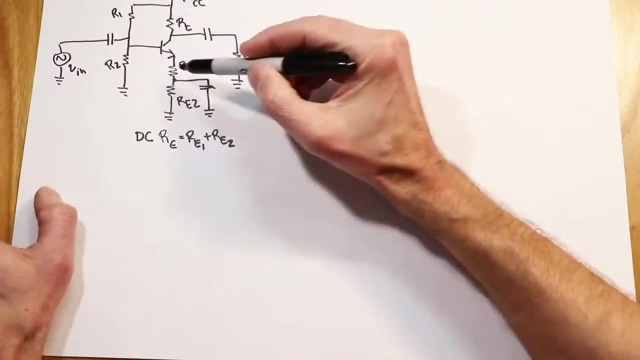 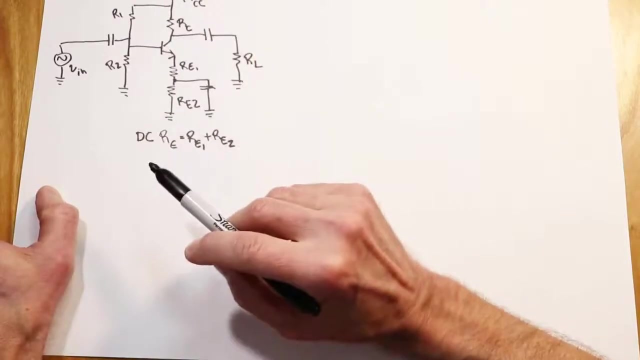 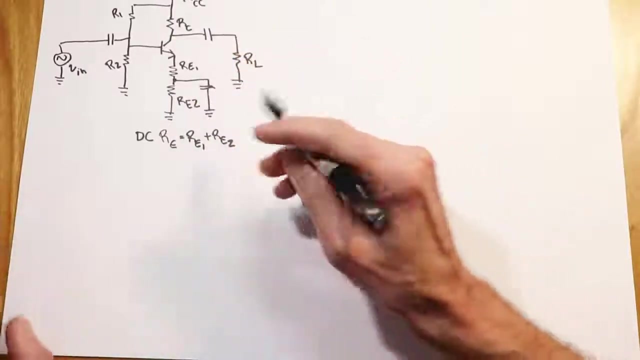 R2, over R1 plus R2 times the power supply That would get us to the base voltage, DC base voltage. Subtract off your 7 tenths on the base emitter and what's left is of course going to drop across the combined emitter resistance, this capital RE over here That will establish our emitter current. Now we need the emitter current because for the transistor model, you might recall, the internal value of dynamic emitter resistance is a 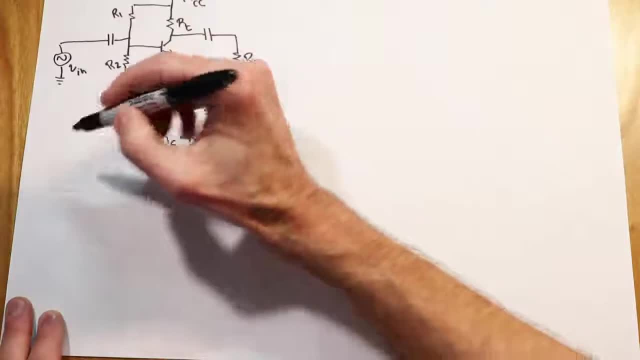 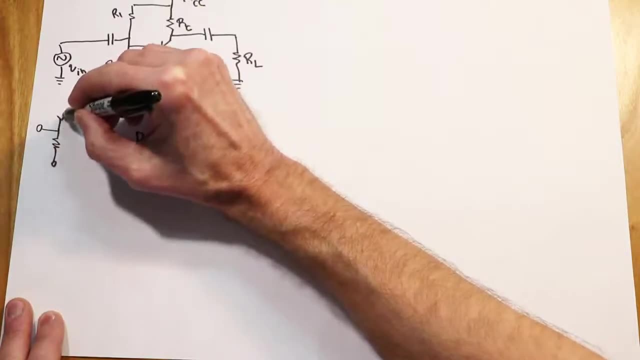 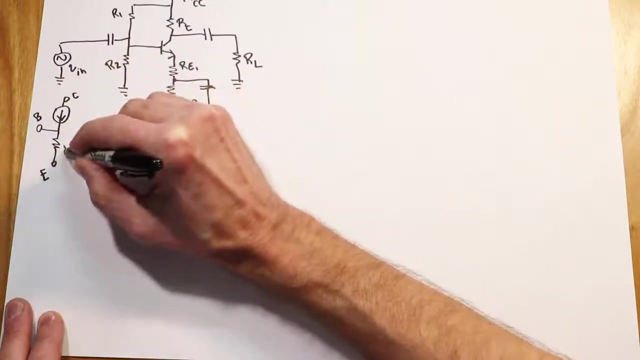 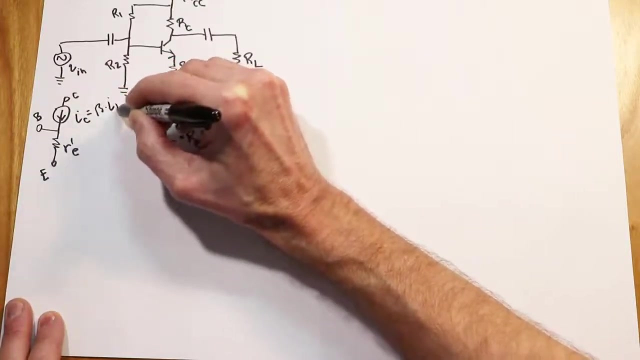 function of emitter current, the DC current. Our model looks something like this: Collector base emitter. So this is the R prime E and we have AC collector current of beta times, IB R prime E. very important, this is a function of the design of the transistor. 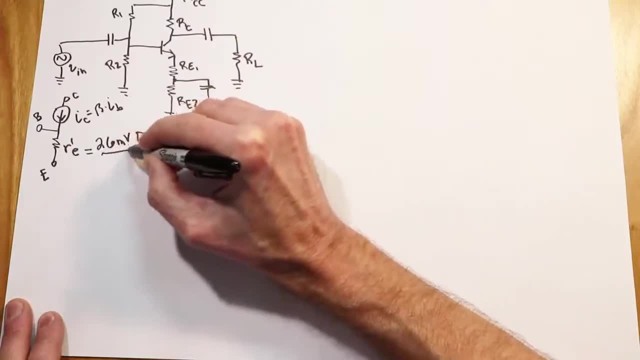 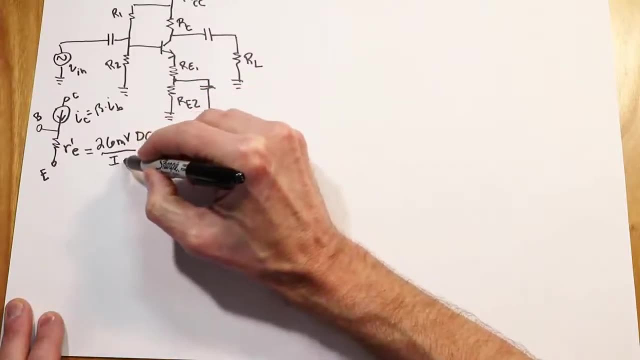 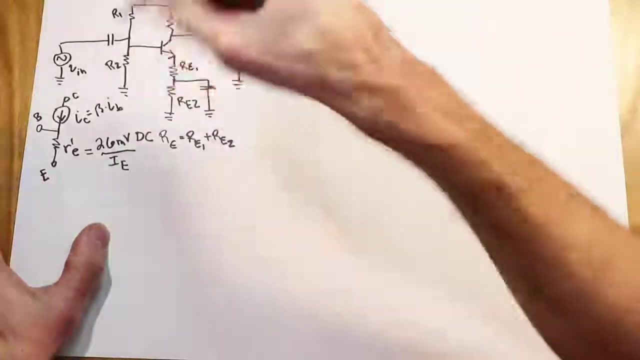 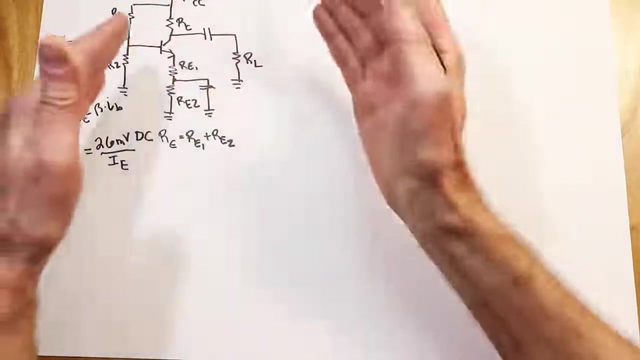 26 millivolts. we take that as a constant at room temperature. It is a function of temperature: 26 millivolts at room temperature divided by IE, and that will get us the value of our prime E. All right now, having done our DC analysis and having obtained our prime E, what we would like to do is turn over to an AC equivalent circuit. 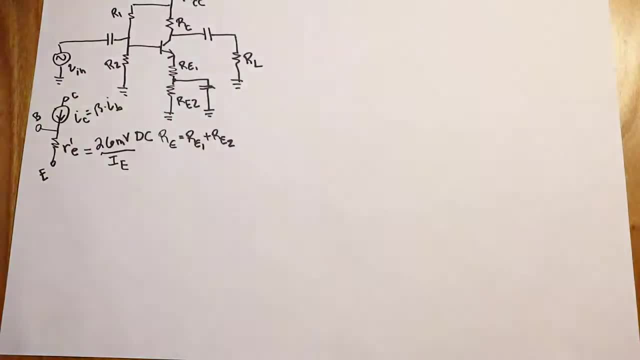 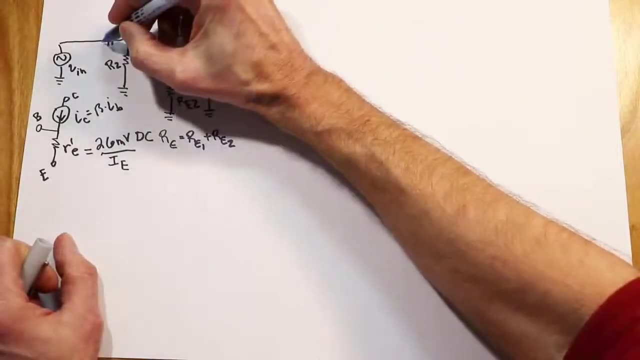 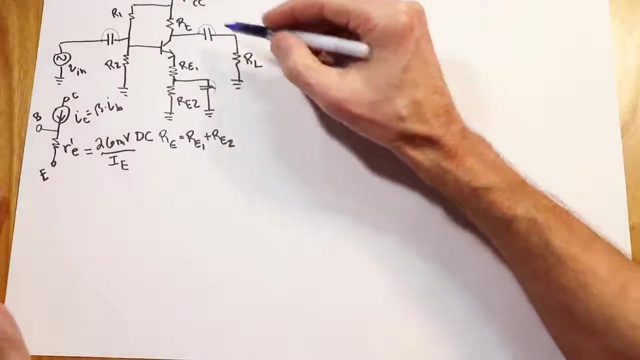 All right. so now for the AC. what we're going to do is we are going to short out these capacitors right Now. their capacitive reactance is going to be small enough so that we can just call them shorts. In other words, by small we mean relatively small compared to the surrounding resistor values. 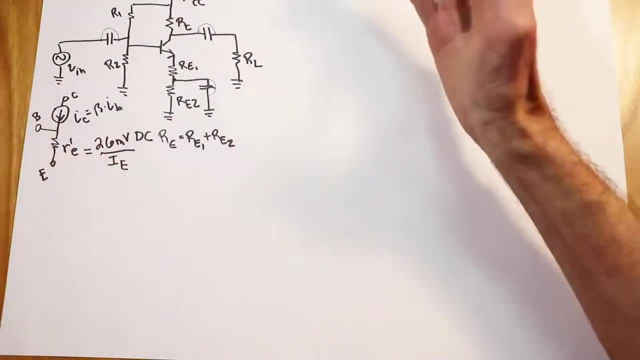 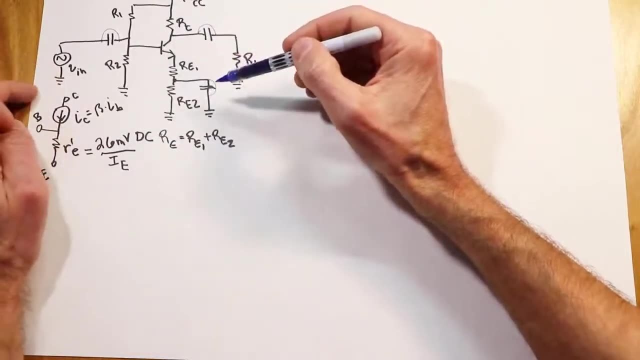 All right, we're not saying they're literally zero, but they're small enough that we can call them or approximate them as shorts. Now, effectively, we're doing superposition here. So, considering the AC source, remember when you do superposition, all other sources are replaced with their ideal internal impedance. 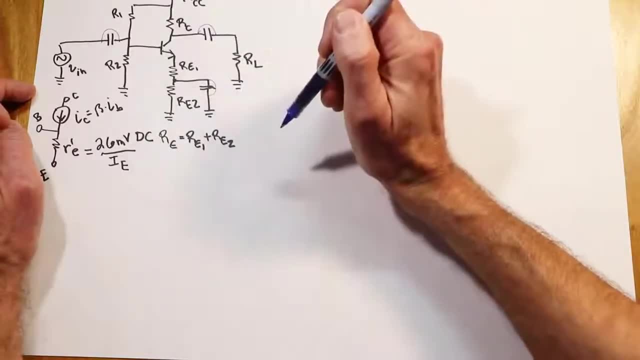 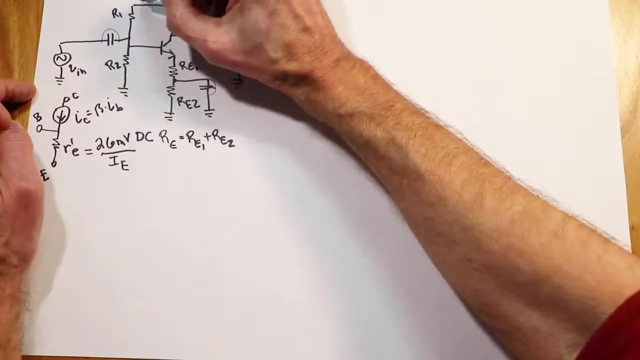 The source that we have here, of course, is the power supply, So we replace that with its ideal internal impedance, which would be a short, because it's a voltage source. So this point basically goes to AC ground. All right, now we're going to redraw this. 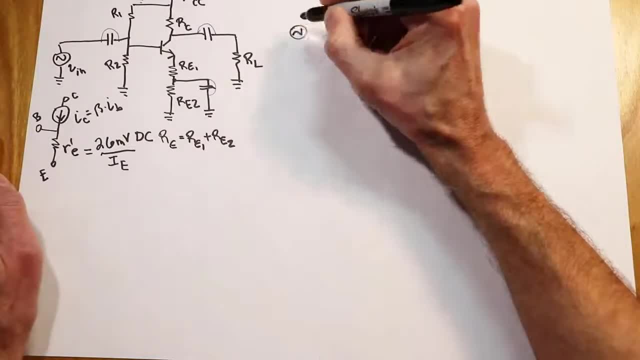 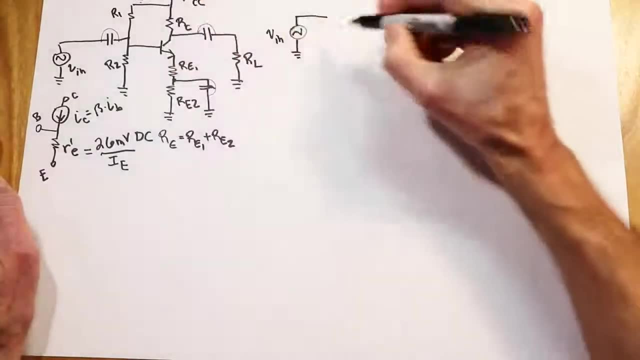 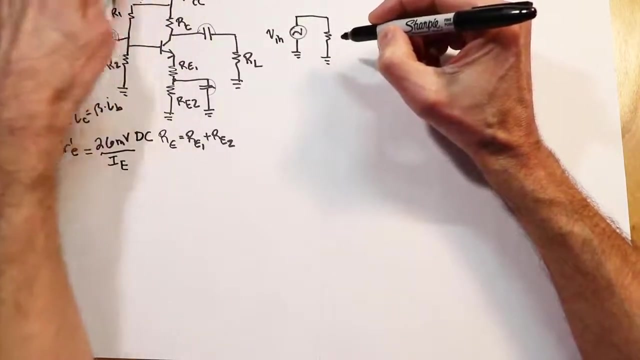 So here is our AC source. All right, that's our VN. Then we see these two resistors, R1 and R2, right. R2, obviously going straight to ground. R1 going to ground because of the shorted power supply. 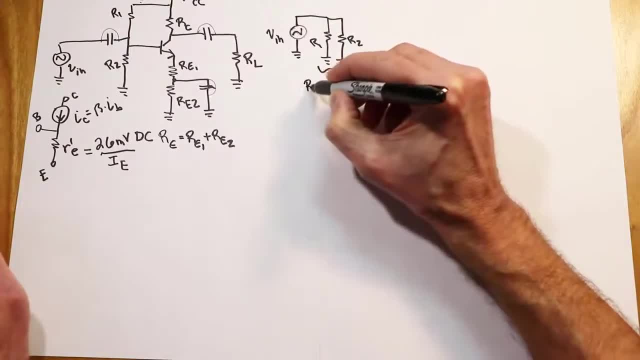 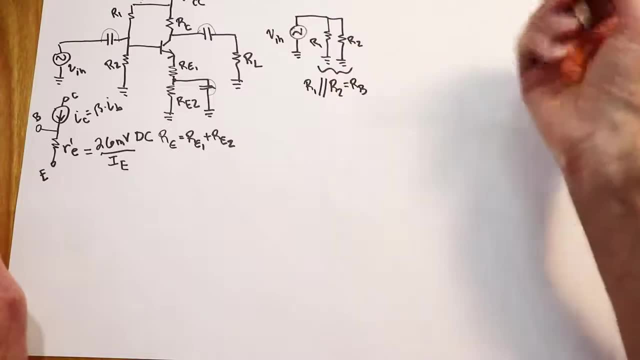 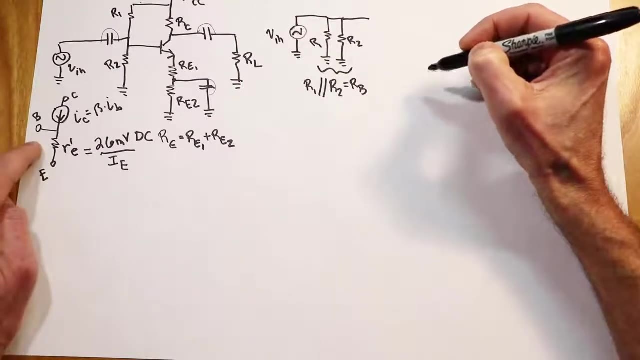 Obviously, we can put those two things in parallel. right before we continue. We'll just call that maybe RB or something like that, for base resistance, base bias resistance. Now we come into the transistor and we're going to replace the device with our AC model. all right, 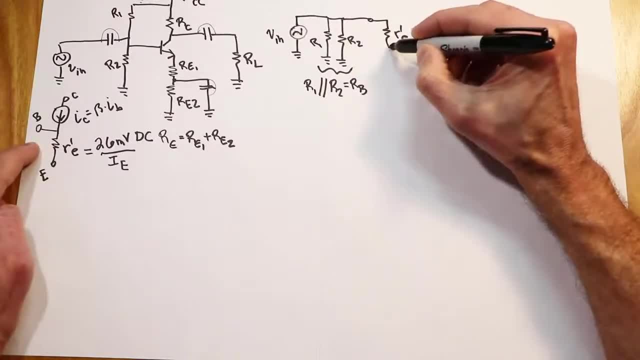 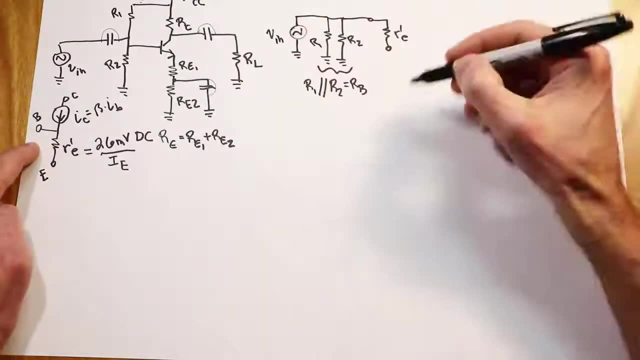 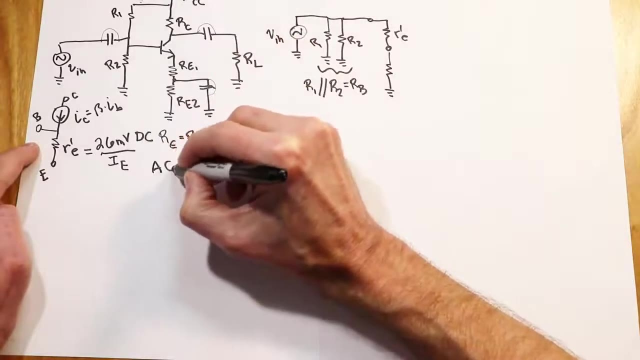 So here's the R prime E value, There's the emitter. Now we have the short here. so this point is AC ground. So we see the RE1 going to ground. all right, So we refer to that RE1, the AC case for RE. in other words, the little RE is just equal to R1.. 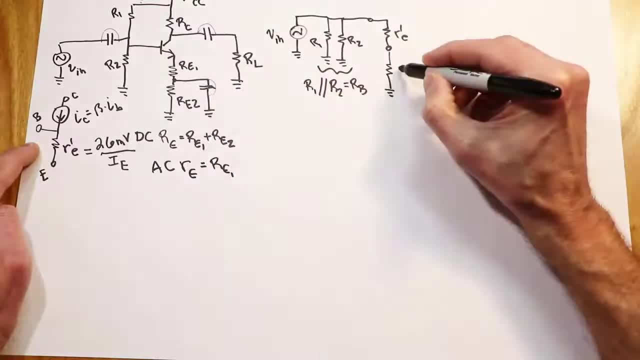 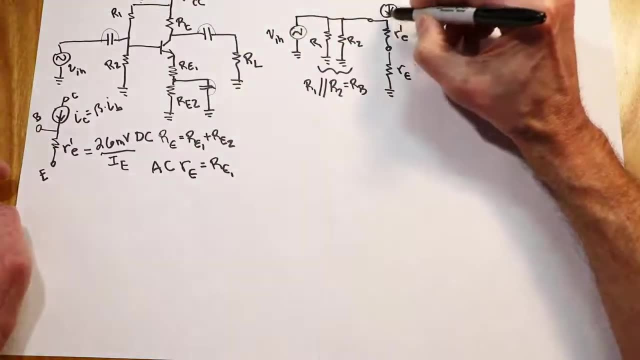 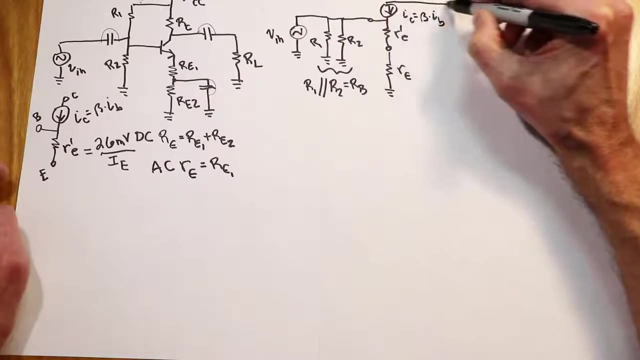 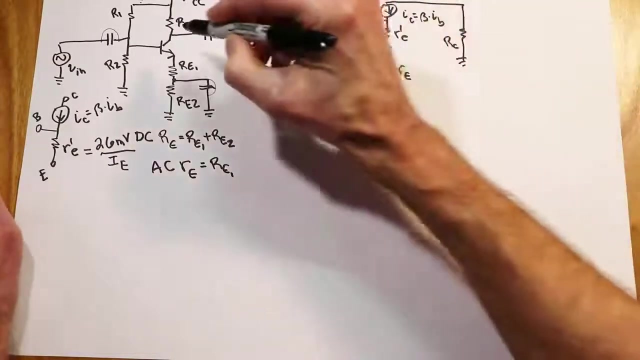 All right, So we have our big RE1.. Okay, So this is our RE over here, And then, coming off the collector, we have our current source. All right, So that is beta times IB. And then we see RC, the biasing resistor, going again to the AC ground from the power supply. 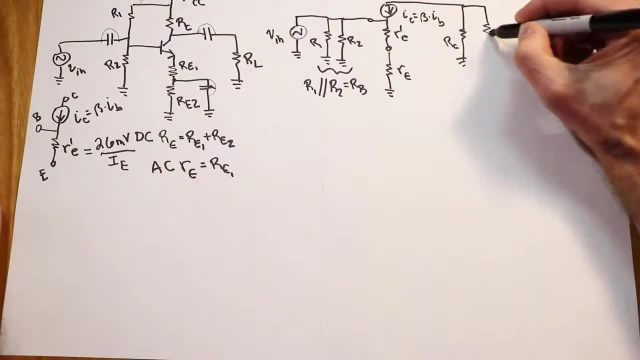 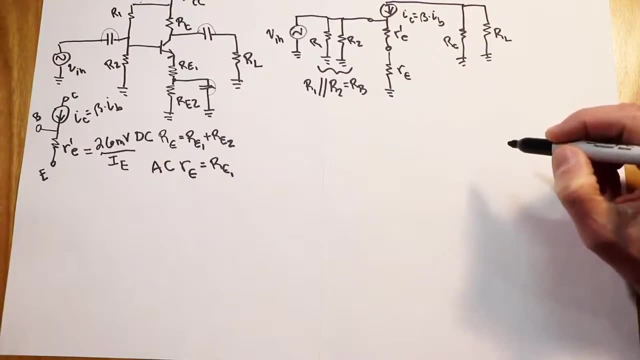 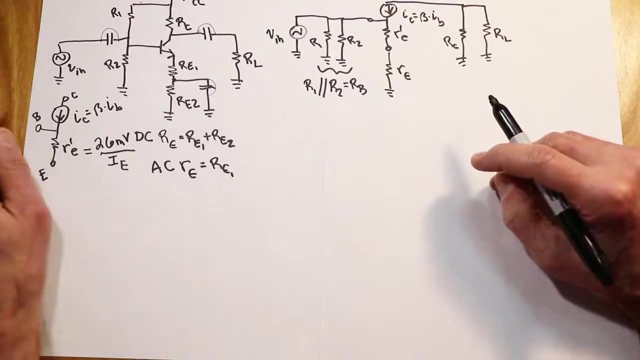 And finally, the output cap is shorted And we have our load resistance RL. Okay, All right. So the three things we are interested in again: the output impedance, the input impedance and the amplification factor. I'm going to grab the output impedance first because it's essentially the easiest one. 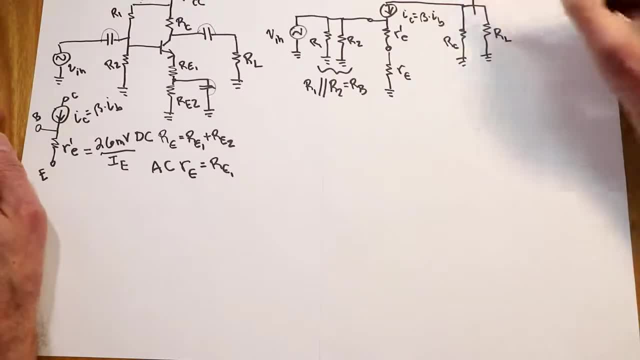 So, essentially, we look back from the position of the load be the load. look back in this way. What do you see? Well, we see this RC, obviously, And that winds up being in parallel with the impedance looking in at this point, which is essentially the internal impedance of this current source. 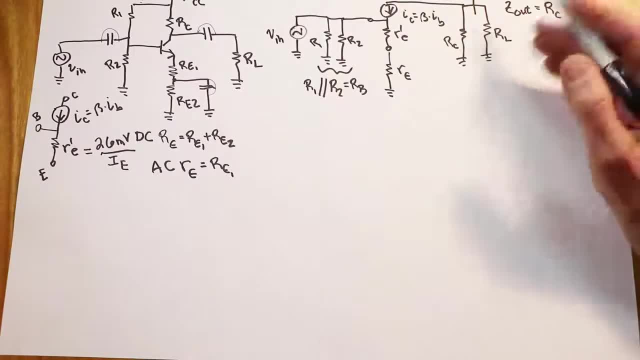 Well, ideally that's an open, All right. In reality it's going to be a very large value, hundreds of K ohms, maybe megaohms, all depending on the transistor, But it's going to be a very large value. 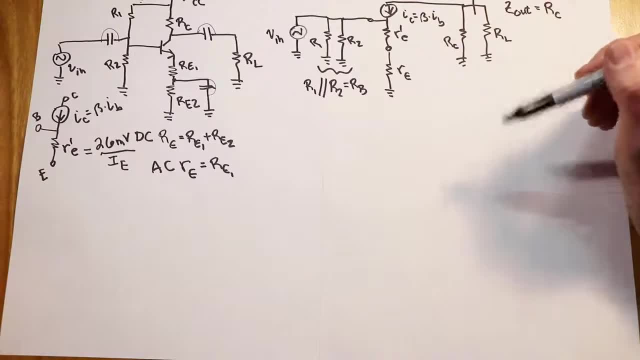 And for typical sort of biasing resistors that we would use, it's large enough to ignore. So we can just say that Z out is whatever it is, Whatever that biasing resistor is, And we're done with it. Okay. 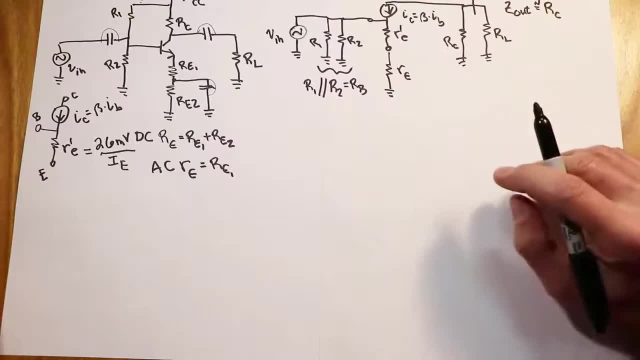 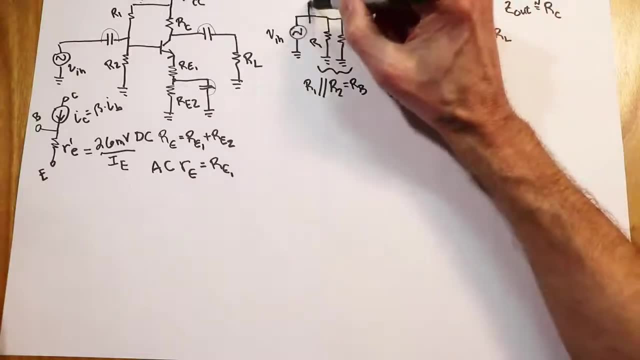 Beautiful. Okay, Now continuing along as long as we're on the impedance part of it, let's take a look at the input impedance. Okay, So the input impedance is back here. In other words, what does the driving source see? 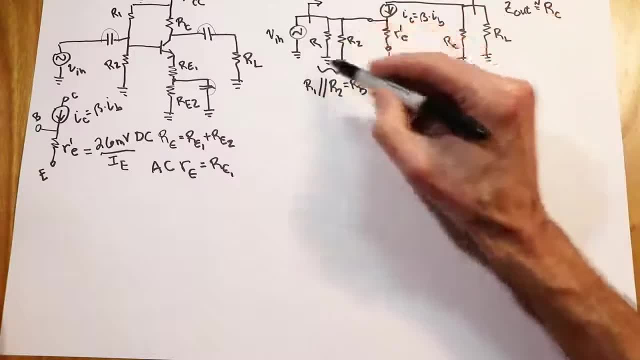 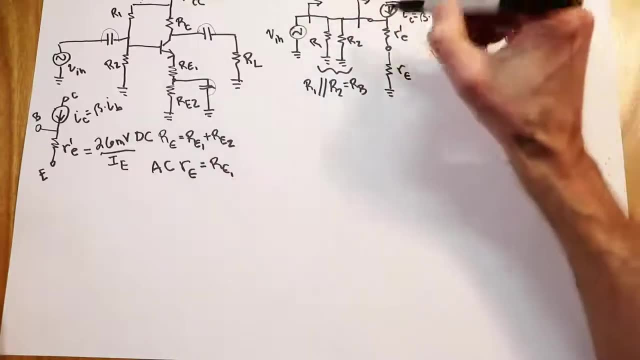 Okay, Well, that is really two parts. You can see that we have this RB value And that is going to be in parallel with whatever the impedance is looking in. What are the impedances? looking into the base, All right, Which we will call Z in base. 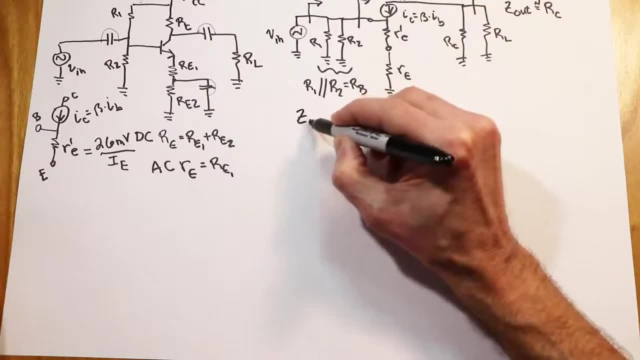 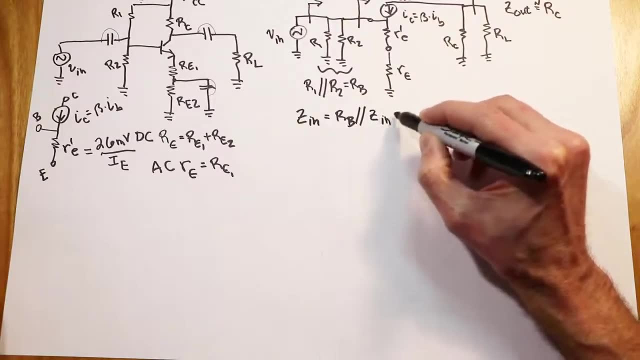 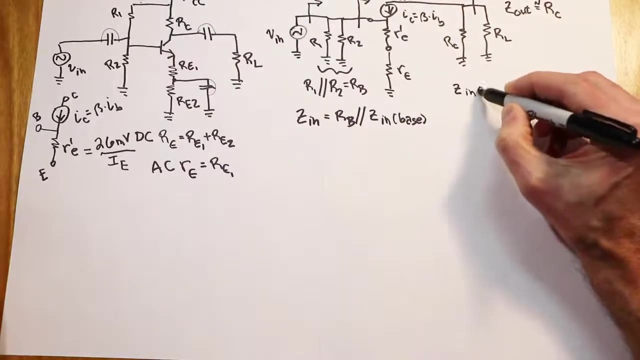 All right. So Z in? is this RB in parallel with Z in base? Now we have a new question to ask: What the heck is Z in base? All right? Well, by definition, Z into the base would have to be the voltage. 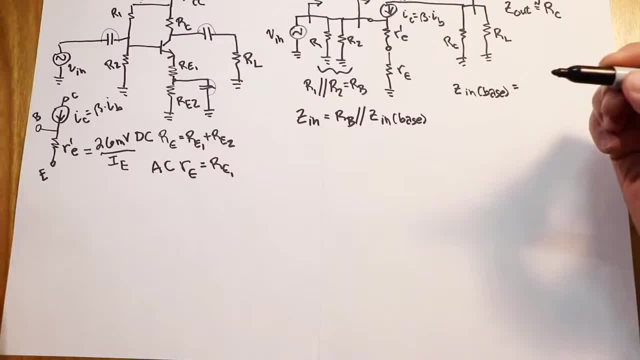 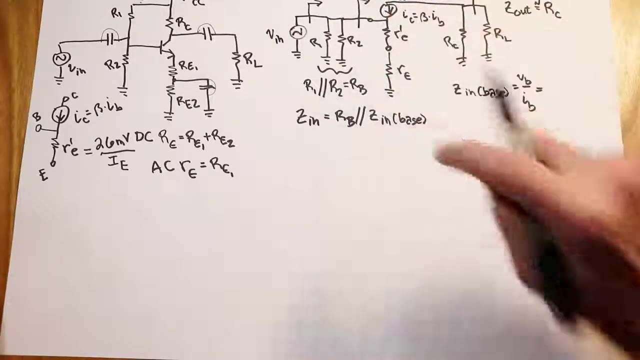 It would have to be the voltage at the base divided by the current. going into the base right: VB over IB. Well, what is VB? All right, This is VB right here, base to ground. Well, you notice that that's the voltage across the biasing resistor RE1.. 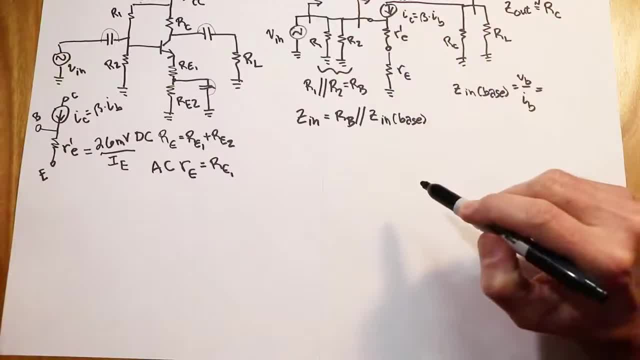 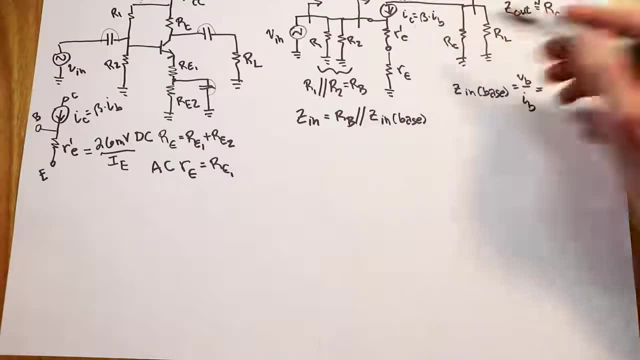 In other words, our little RE and our prime E. All right, How do I describe that? in terms of Ohm's law? It's that resistance times that resistance, That resistance times, the current through it, which is IE. IE and IC, of course, are nearly the same size. 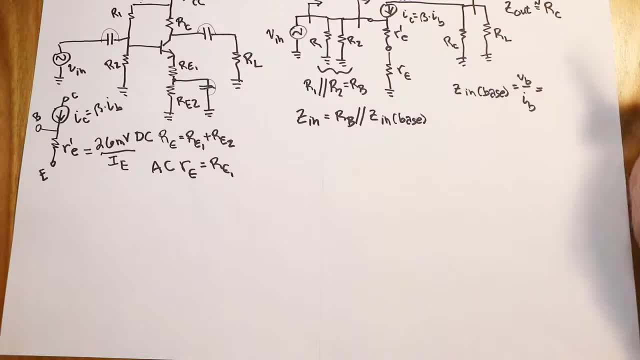 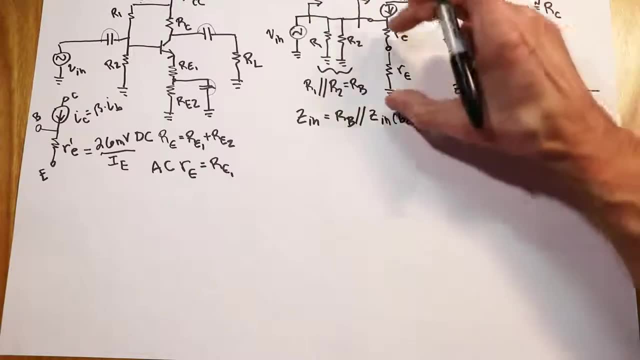 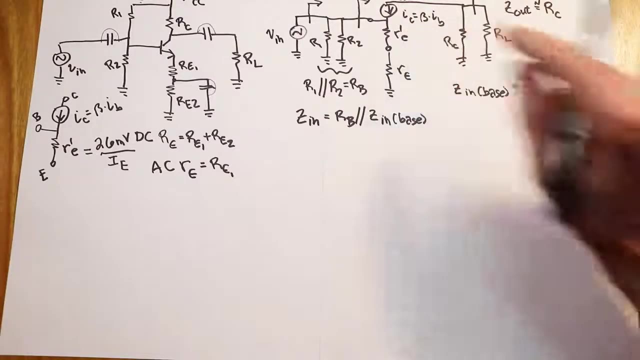 And I'm going to write this in terms of beta times, IB. Why? Because then I'll be able to cancel out the IBs. So we will say then that VB is this potential, which is the current through it, IE, which is approximately equal to IC, which is equal to beta times, IB times, that impedance right. 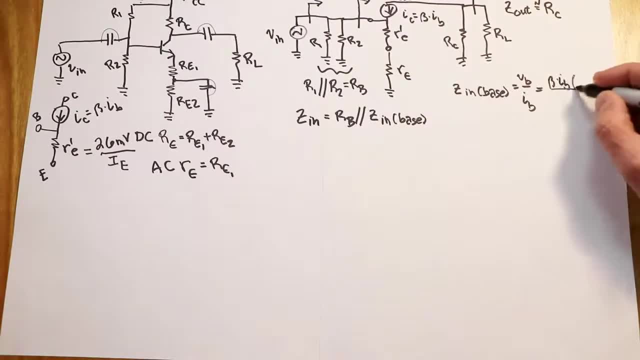 So that's beta times, IB times the quantity R, prime, E plus RE And that's divided by IB. So those IBs cancel out And we see that Z in base is just equal to beta times, the resistance that's sitting in the emitter right. 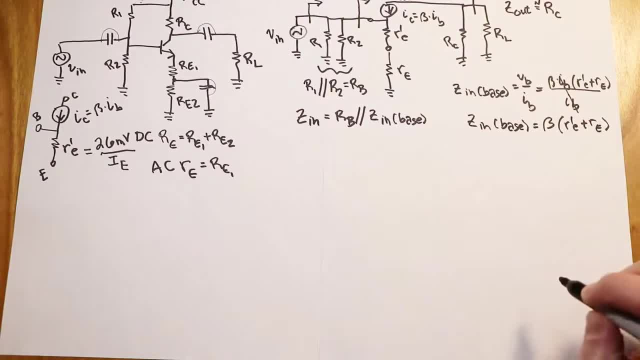 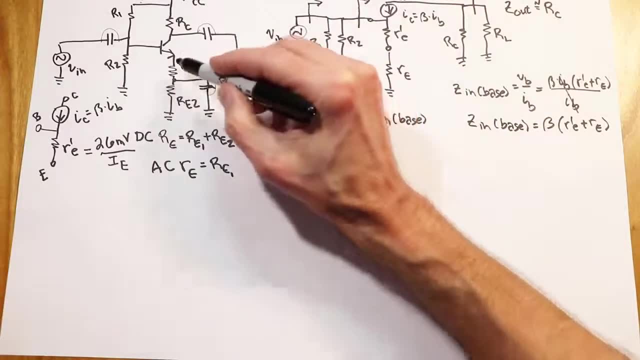 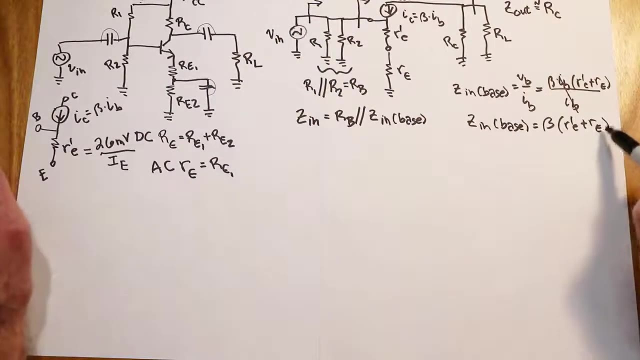 R, prime, E plus RE. All right, If we didn't have this split, in other words, if we just had the one resistor here and the cap just went up right to the emitter, then RE would be zero, right? This would be sort of a special case- you could think of it- where RE is zero. 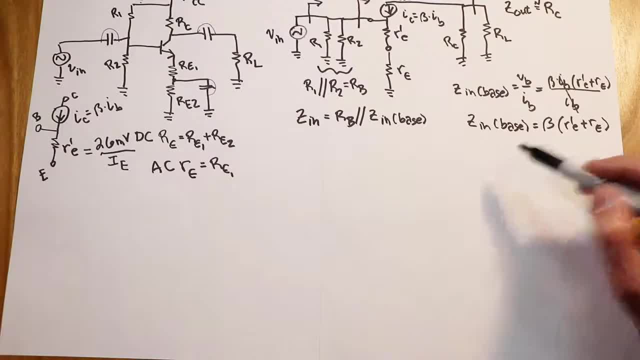 Your Z in base would be smaller. right Typical values, RE is going to be a lot bigger than R, prime, E, So it tends to dominate in usual circuits And that tends to increase your Z in base, which of course, back here would then increase your Z in. 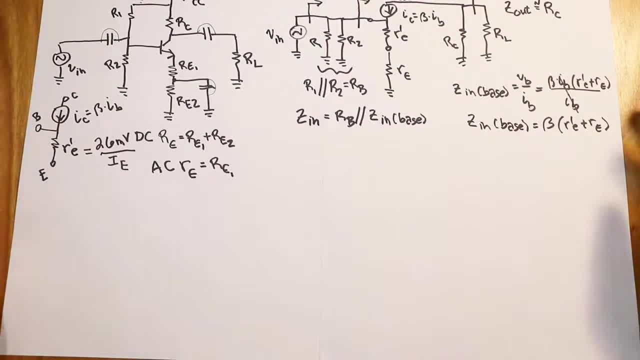 High input impedances For general purpose amplifiers, like audio amplifiers, is generally a good thing, Because that means you're not drawing a lot of current from the driving source. all right, All right, that's two down, one to go. 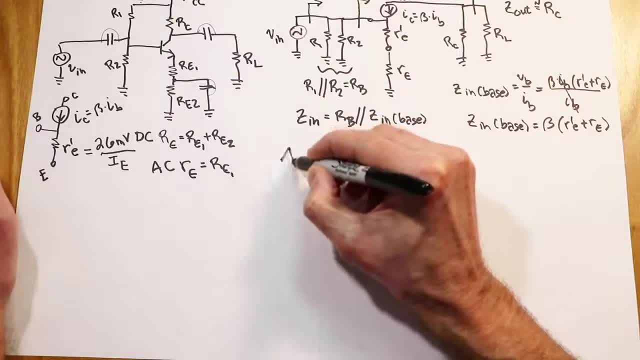 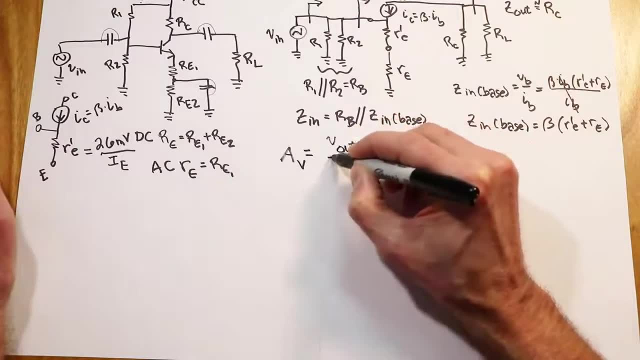 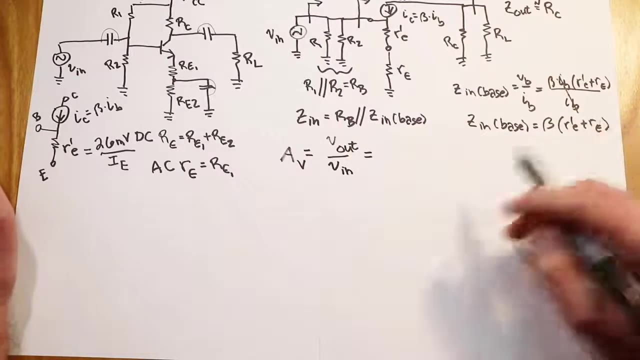 That's the voltage gain, the amplification factor AV. Well, that's essentially your output voltage divided by your input voltage. Now there's two ways we can go about this. We can look at what's called unloaded gain And we can look at loaded gain. 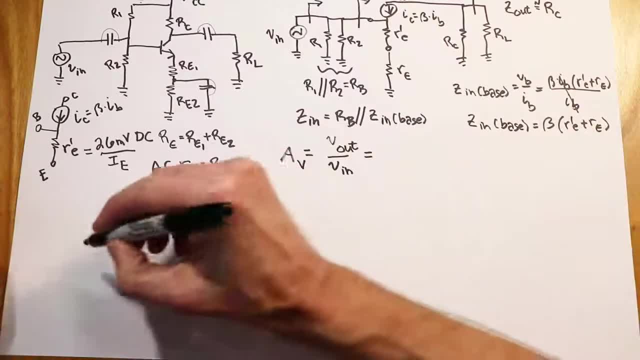 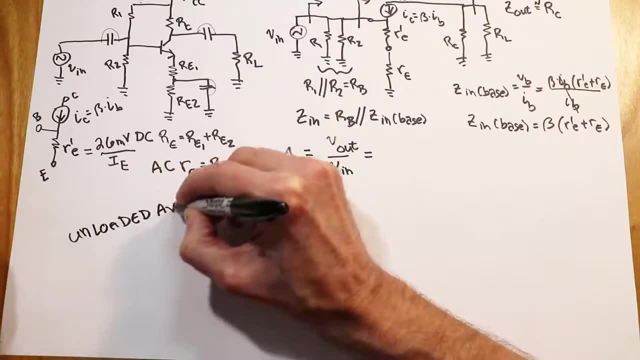 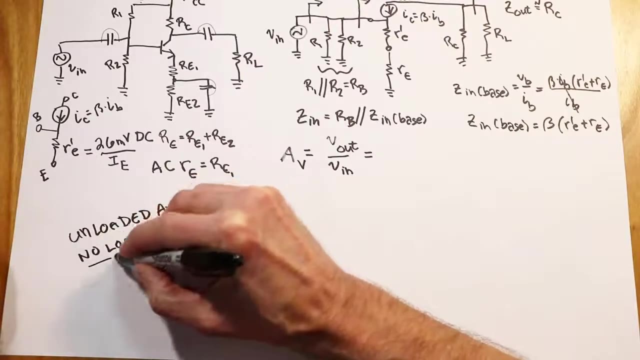 So unloaded gain is the maximum gain that you can get, okay. Unloaded literally means without load, okay. So loaded AV, no load okay. So we just unhook it. it's gone. it's history all right. 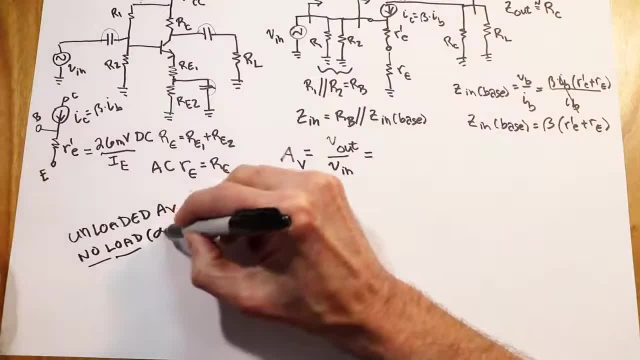 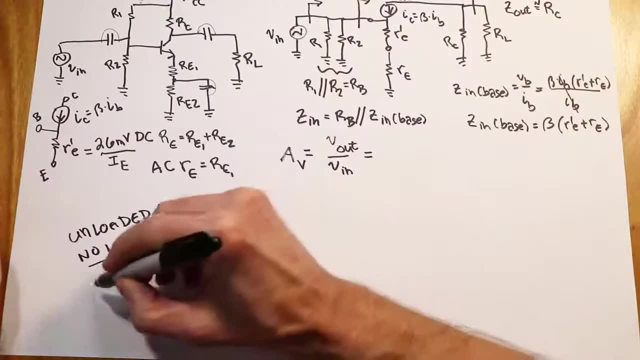 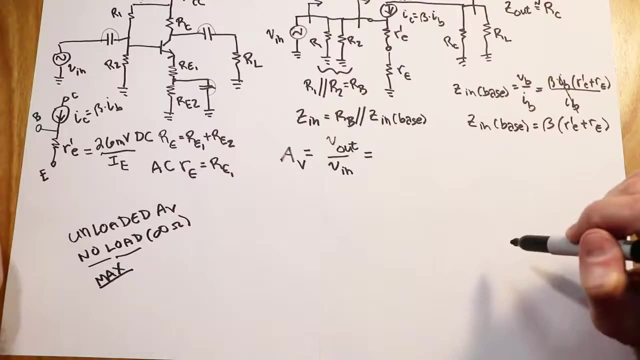 Think of it as infinity. This is the maximum gain You can never hope to get out of here. all right, In the loaded case, you know, we do add on an RL and that will decrease the total impedance seen out here. 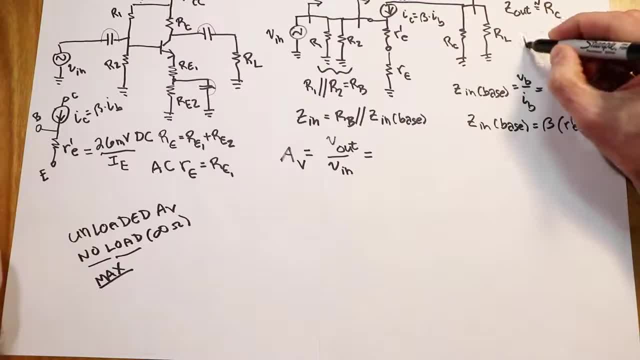 What I need to consider is the value for little RL, which we sometimes refer to as little RC, the AC values. Either way you do it, it's big RC in parallel with RL. okay, You can see, those are just directed, They're not directly in parallel. 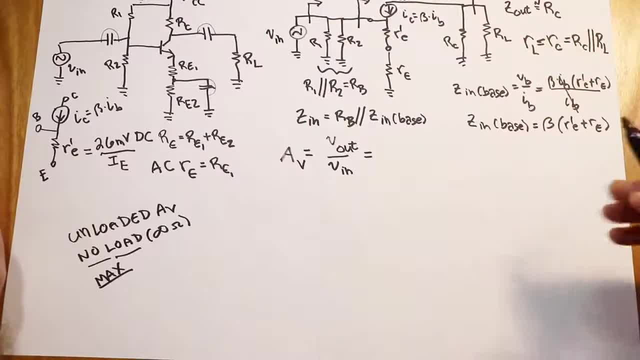 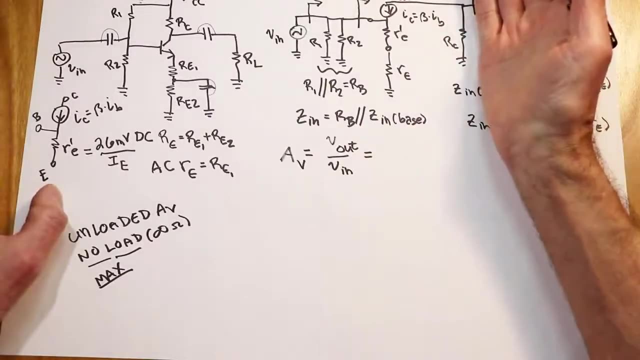 Essentially, what we're going to do is the same computation, either with just the big RC, in other words unloaded, or with the parallel combination. okay, So let's just look at the unloaded gain first. What is my output voltage? 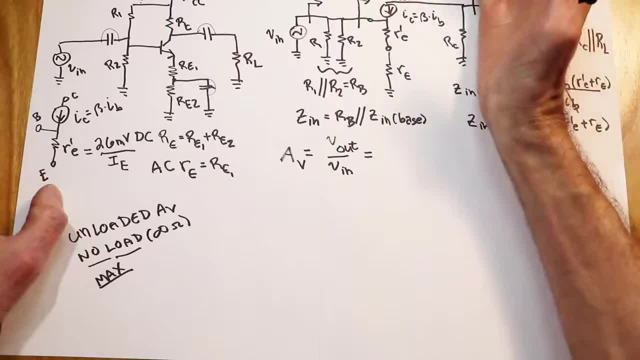 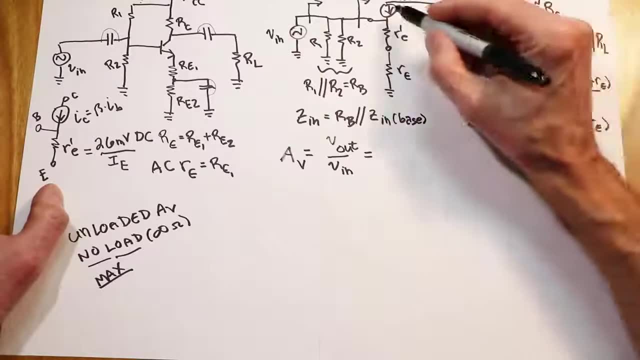 Well, it's the voltage across this RC. right Again, we're pretending that's gone. How do I write that in terms of Ohm's law? Well, this resistance times the current through it. What is the current through it? 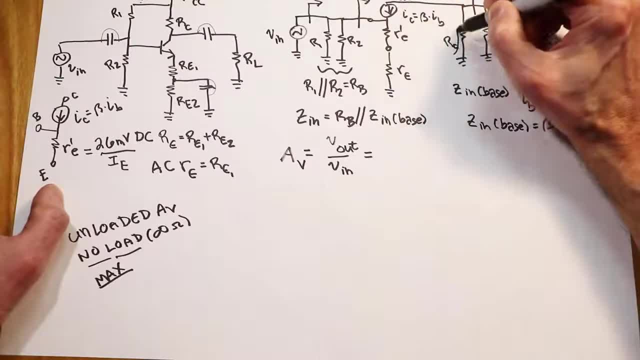 Well, it's controlled by this current source, So that current's coming up like this and that produces a polarity on here of plus to minus, bottom to top. So your output point is negative with respect to ground. So this is going below ground. 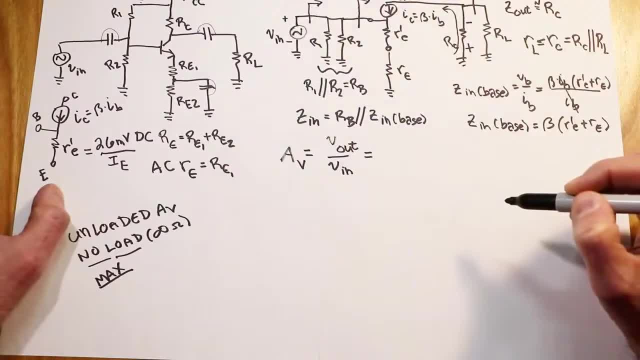 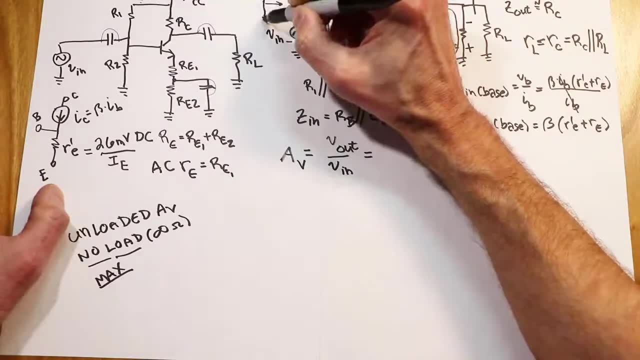 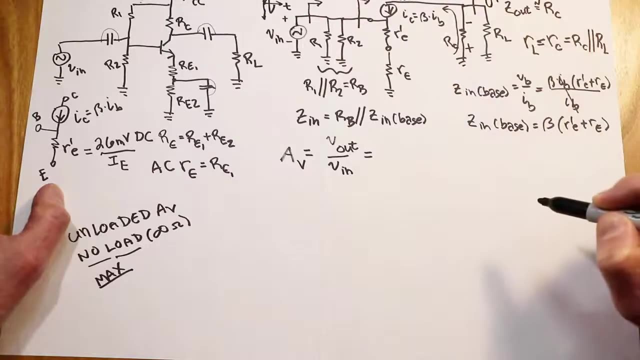 and this would be the case for a positive input polarity right. What does this mean? Well, that means that if your input polarity is a normal sine wave, like this right, then your output polarity would be going like this: It's flipped upside down. 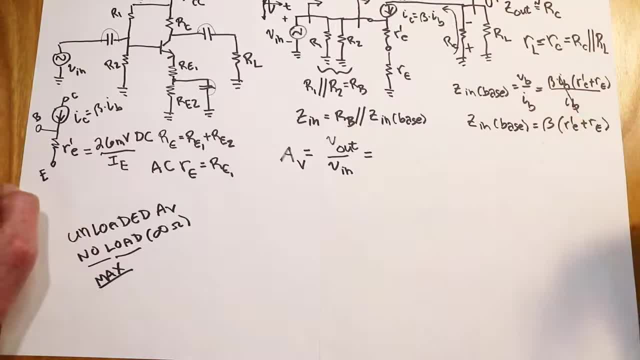 Now, in many cases that doesn't make any difference. If you, for example, flipped the phase, you flipped the signal coming out of you know something simple like a walkie-talkie, an intercom, whatever table radio. 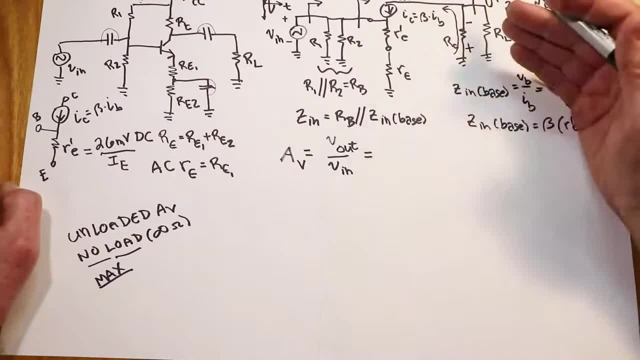 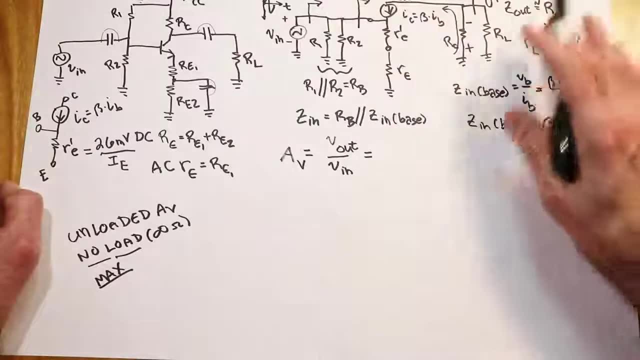 you really wouldn't be able to hear the difference. okay, In some applications it makes a big difference. You have to maintain, You have to maintain the correct phase. But be that as it may, we simply would know that the output is negative. 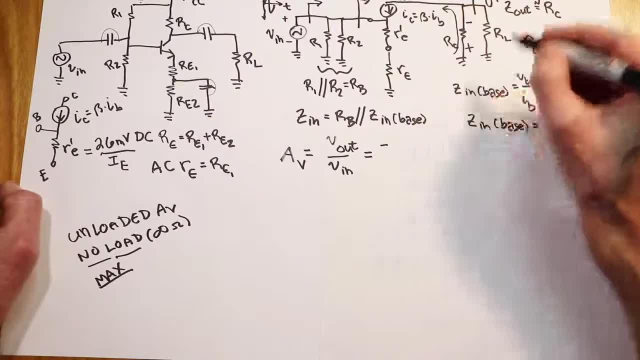 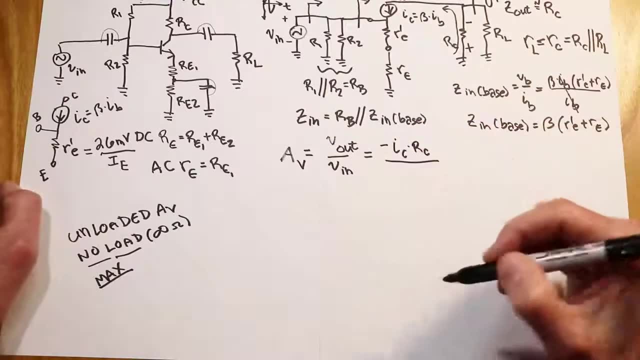 So I'll just say: well, that's a negative RC times the current right, So that's just IC times RC. How do I write my input voltage? Well, we've actually already done that. looking at the input impedance. 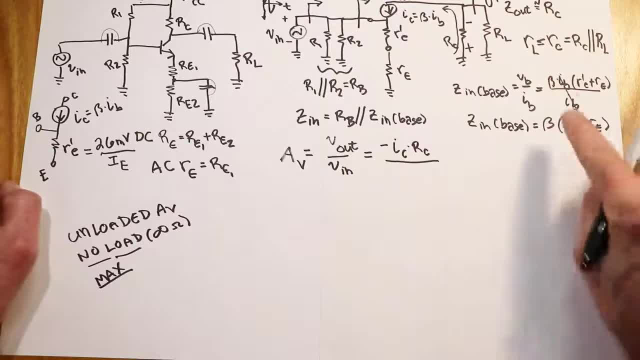 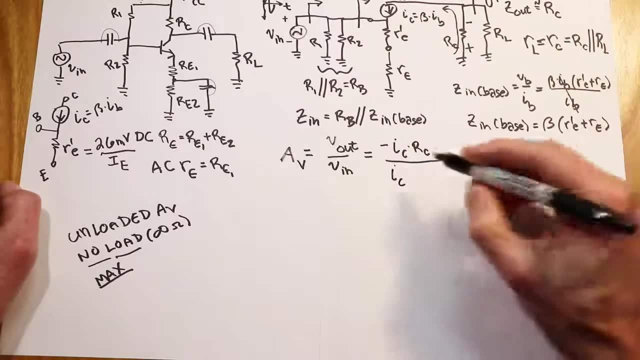 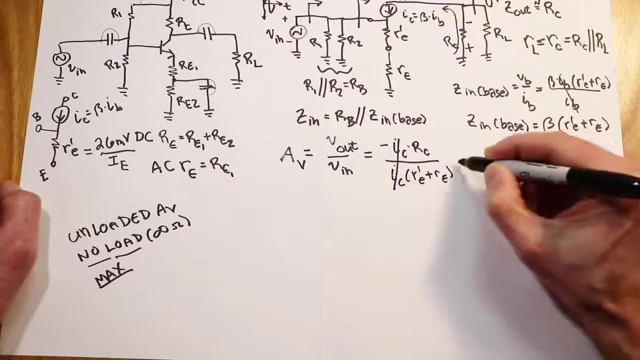 So the input voltage is this: VB again okay, which we know is beta, IB or IC. So that's this: VB times the R prime, E plus RE. Once again, those currents can cancel out and we wind up with a negative RC over R prime, E plus RE. 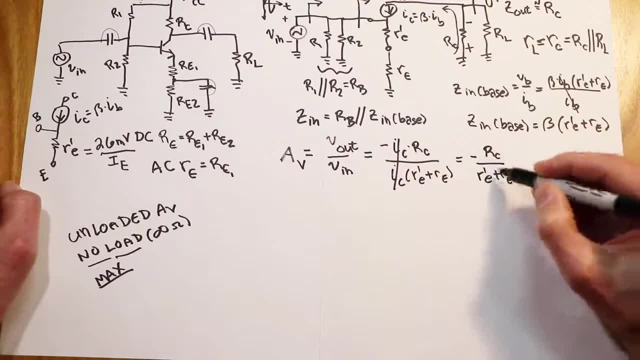 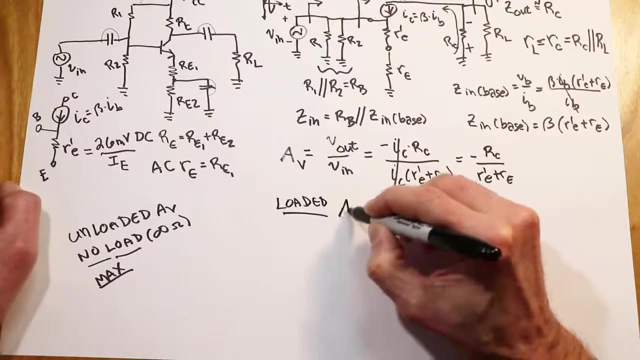 So as long as that resistor is considerably larger than these resistors, we'll get a much bigger output voltage than we have as an input voltage right. Wonderful For the loaded gain. the only difference is the value that you're going to use for your load right. 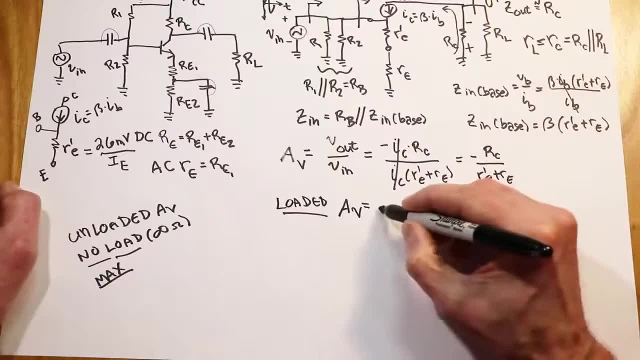 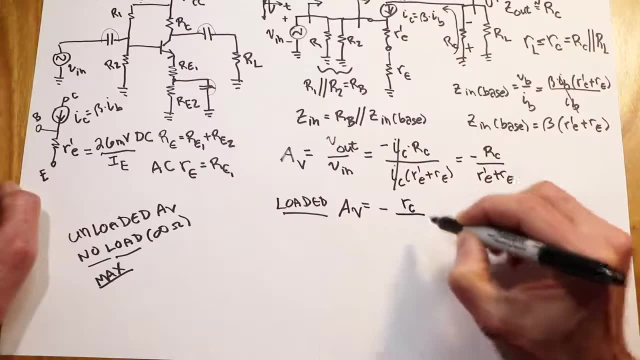 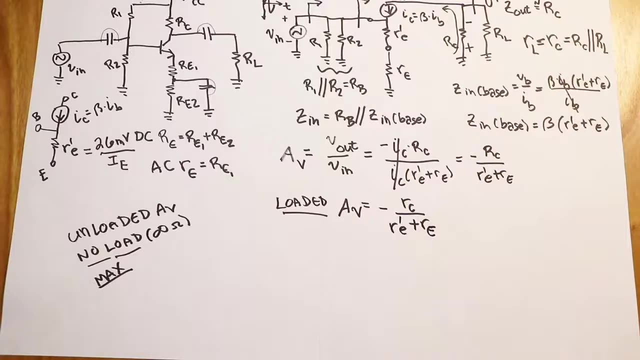 It's going to be little RC or little RL, whichever you prefer, instead of the biasing resistor RC. And the question might be well, why do I calculate both of these things? Well, you know, if I just had the one load, 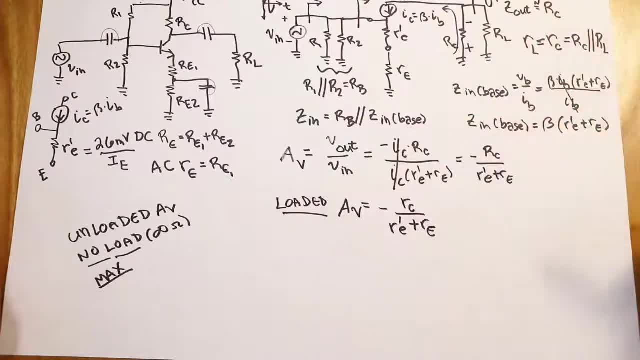 all right, I've got a fixed load out here. we would probably just calculate the loaded gain and be done with it. On the other hand, if we're changing what the load is, then it actually makes sense for us to figure out the unloaded gain. 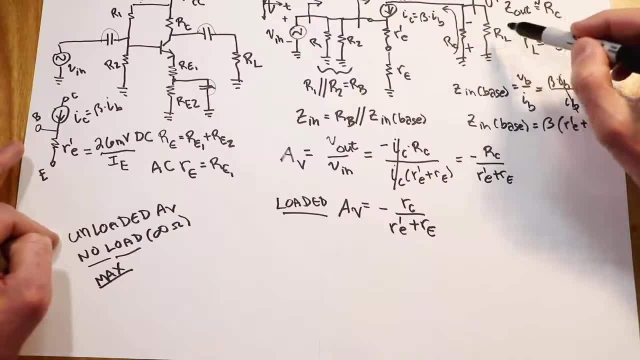 and then we can figure out what the effect is of the load separately. The way we would do that would be through a little voltage divider, Because what we're really saying here is: look, there's an output impedance of RC and we can model this, even though this is a current source. 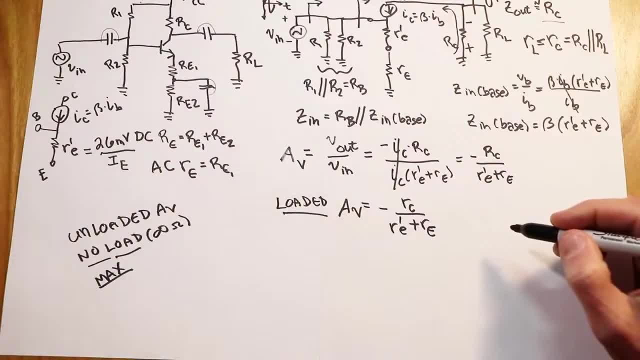 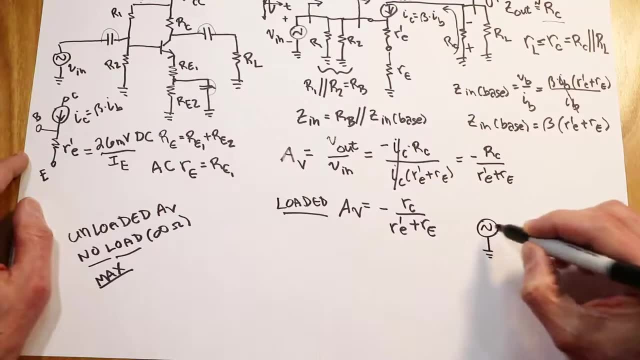 we can still model this as a voltage source, just for visualization, right, Because you know we can't do a source conversion. But basically what we're saying is: this is a controlled source, right, And we convert this. This is a controlled source that's equal to A times, whatever my VN is. 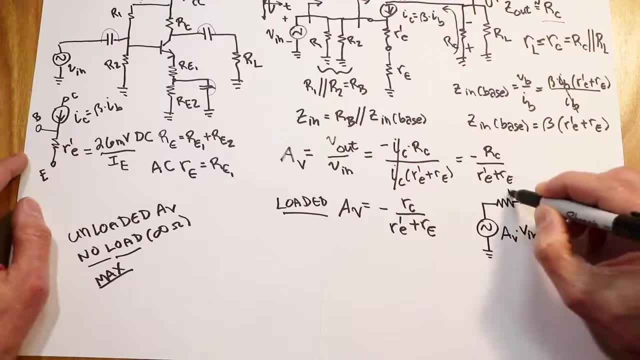 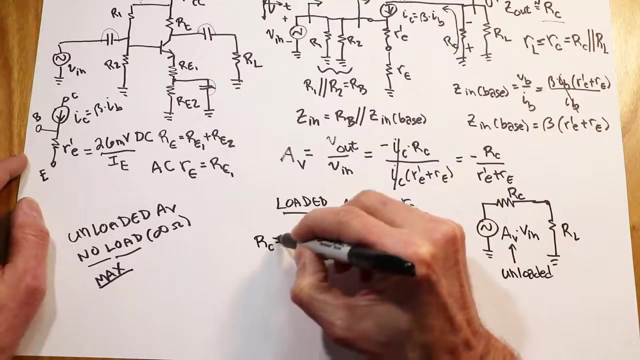 And there's an output impedance that's equal, in this case, to RC, And this hooks up to my load, This being the unloaded gain. So here's an example. Use some easy numbers. Suppose that your RC is 10k ohms. 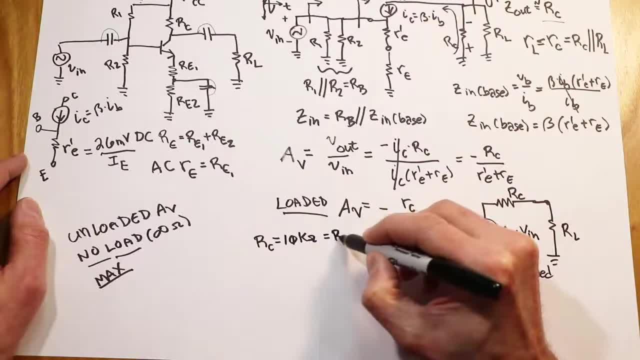 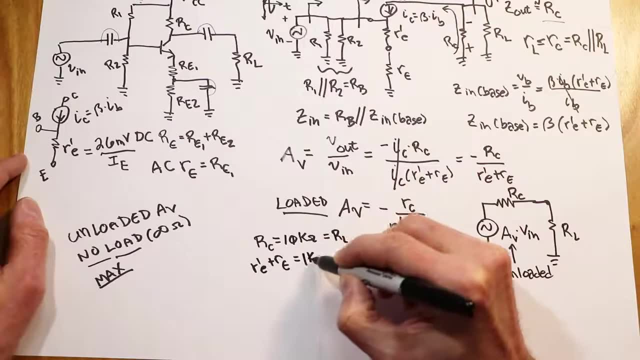 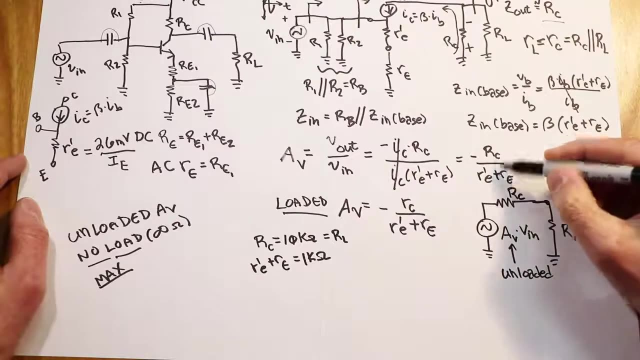 And that's also the value of your RL. Further, let's say, the R prime, E plus RE, works out to a total of 1k ohms. All right Now, if you calculate your unloaded gain, that's going to be 10k over 1k for an inverting gain of 10.. 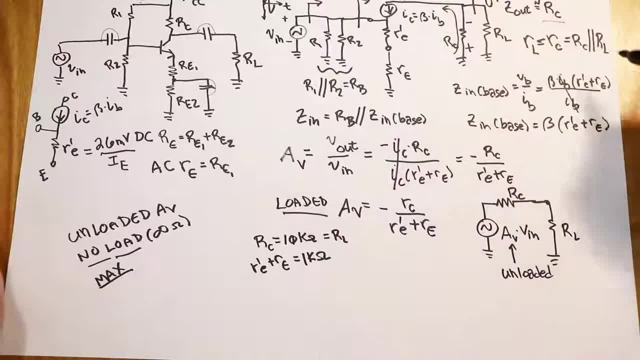 All right. Now, when you throw the actual load on here, right the 10k load, then you'd actually have 10k in parallel with 10k, which is of course 5k. So you'd have 5k divided by 1k. 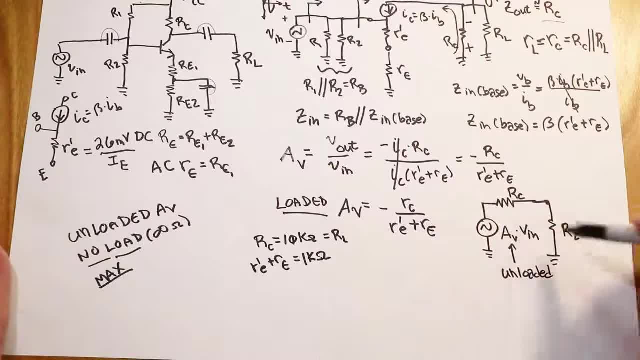 You've got a gain of 5. now, All right, Well, you could do it this way. Say, well, I've got an unloaded gain, I've got an unloaded gain of 10.. And then I have a voltage divider between my RC and my RL. 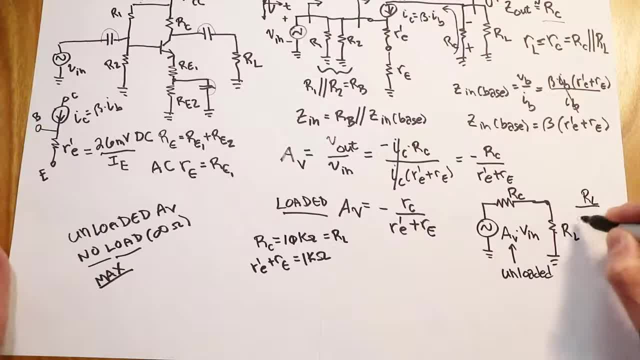 So what is this voltage divider? All right. well, it's the thing you're interested in: RL over the total, RC plus RL. Well, if RC and RL are the same size, all right, if they're both 10k. 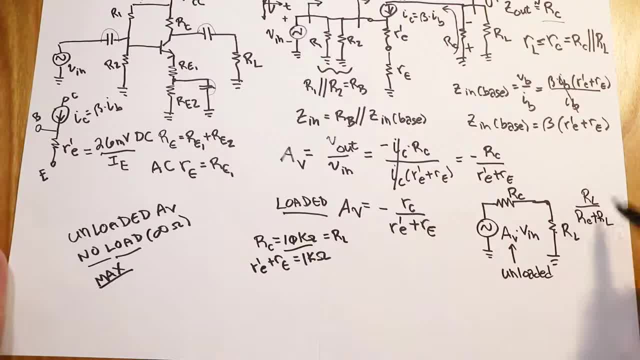 then this is going to be 0.5.. So you have a loaded gain of 0.5 times the unloaded gain of 10, 5, which is what we calculated with the loaded gain. So basically, if you have a situation, 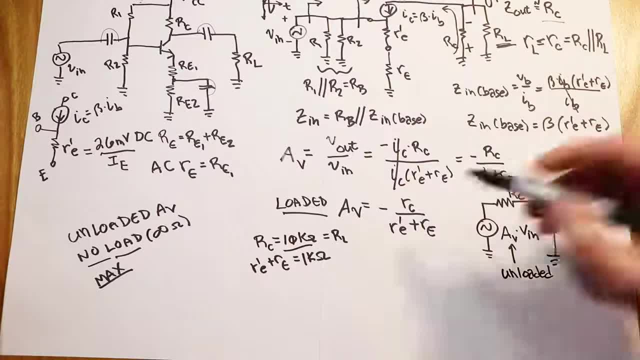 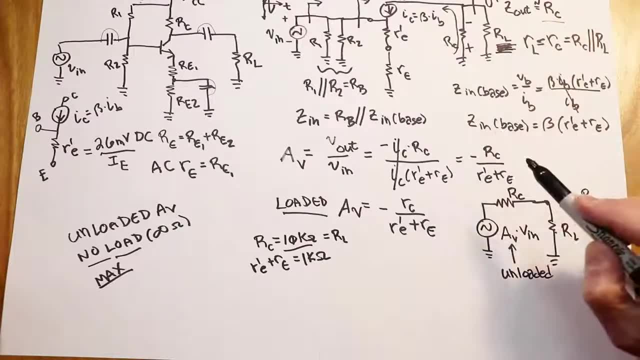 where this load is fixed. it's just going to be easier for you to figure out the loaded gain If this is not a fixed value. if you're going to hook this up to different things, right, different sorts of loads- then it might make more sense to figure out what the unloaded gain is. 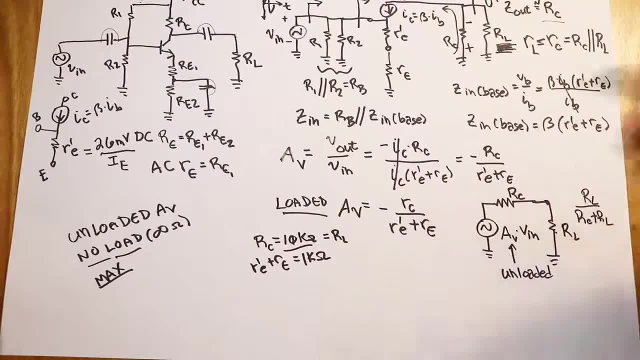 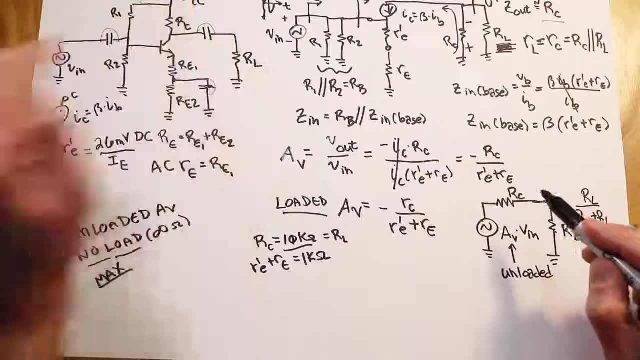 And then you could do this little voltage divider effect to figure out what it is for any particular load impedance. right, You just have to do a little voltage divider effect. Now the same thing can happen at the front end. Now, I'm not drawing it here. 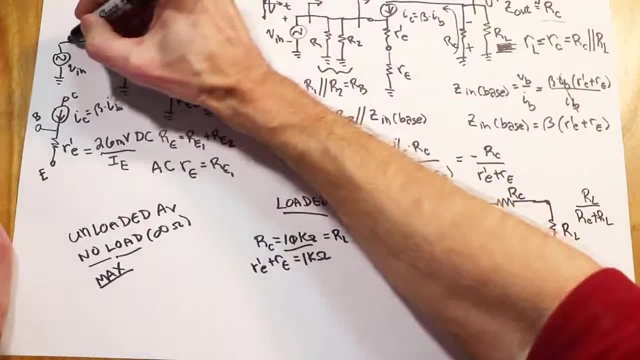 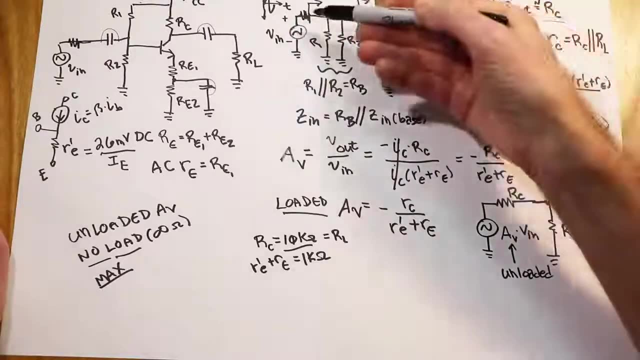 but your source could have an internal impedance associated with it. all right Now. that would appear over here Now in lab if you use a function generator that's 50 ohms And for typical sorts of circuits that we would work with. 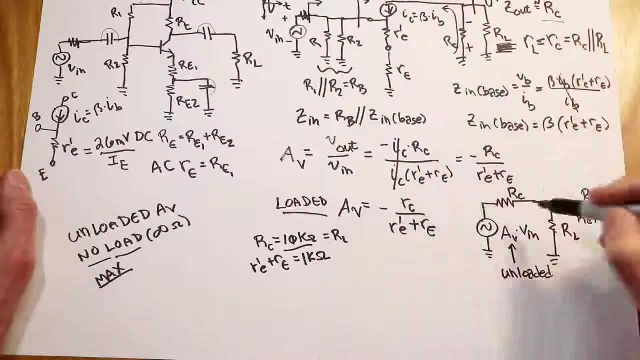 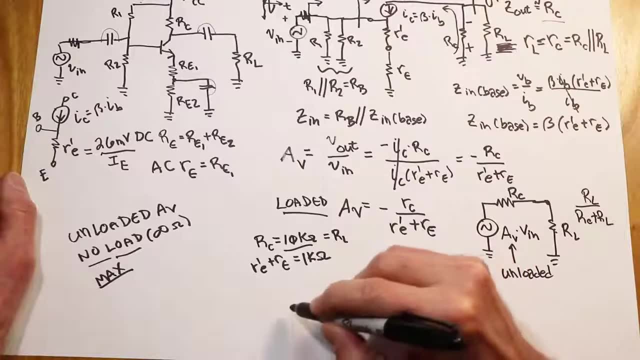 it's small enough to ignore, But in fact, just like there is here, there is a possibility of a voltage divider effect. So here's my input voltage. all right, Here's the source impedance associated with that. I'll call it Rs. 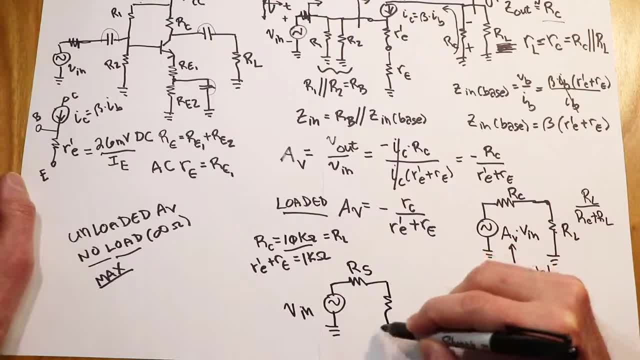 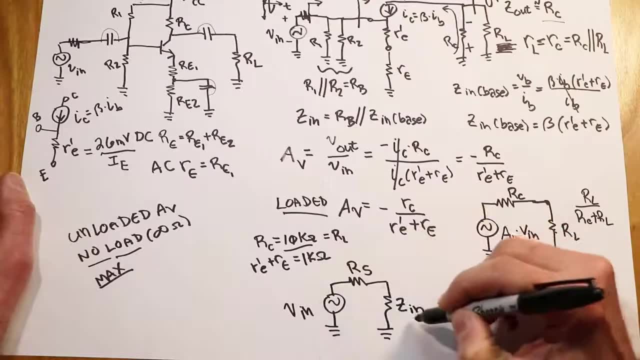 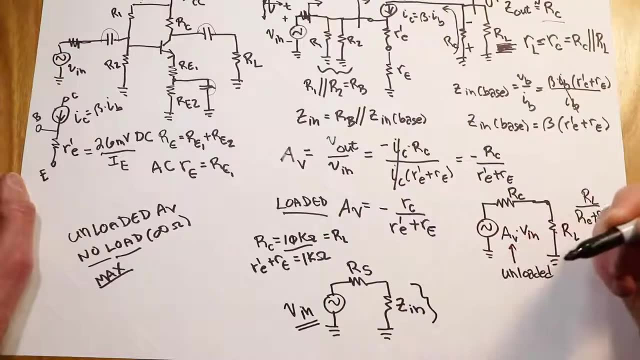 We'll assume it's purely resistive. And then here's your Zn. okay, Now, if Zn is a lot bigger than Rs, virtually all of Vn gets to the input of the transistor. In other words, it actually gets to the base of the transistor. 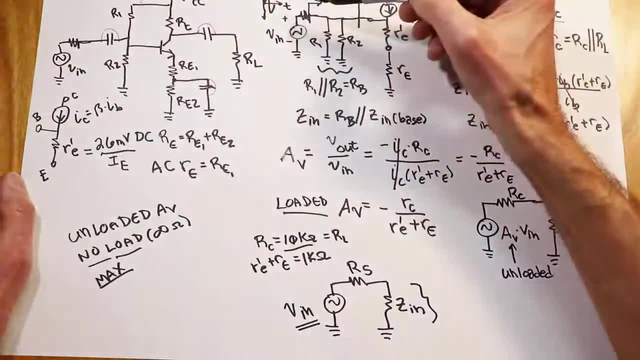 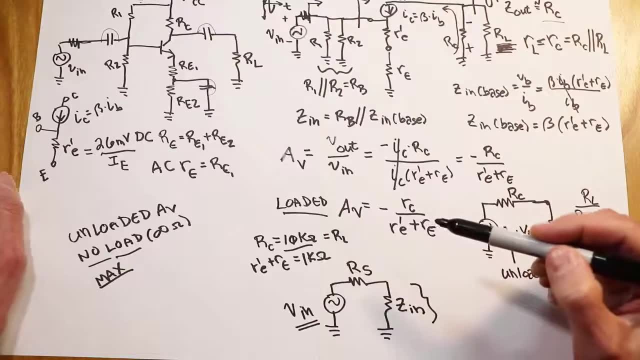 See back here, because we don't have that. we're assuming it's small enough to ignore, then the applied voltage is the base voltage. It's the same thing. But if this internal impedance is pretty large that's not going to be the case. 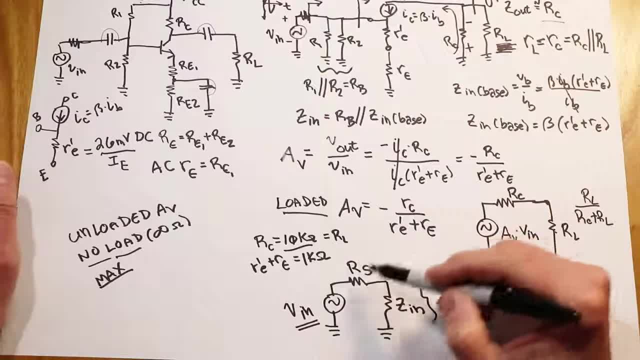 And there are instances where this number can be pretty big. For example, an electric guitar pickup, This could be several k ohms, And if you have a Zn that's just a few k ohms. you know there's a sizable signal mismatch there. 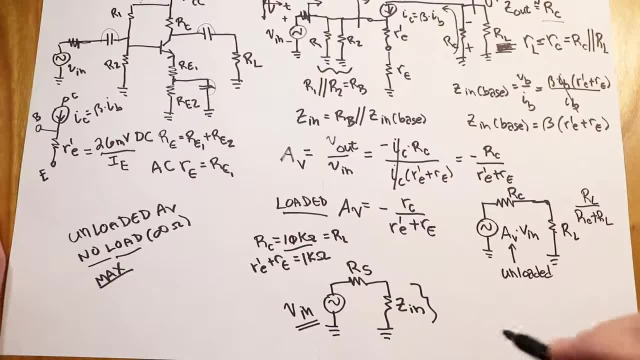 You could lose a considerable amount of signal right. So that little loss, that sort of impedance match or source loss, whatever you want to call it, is nothing more than a voltage divider. So the thing you're interested in, Zn, divided by that source impedance plus the Zn. 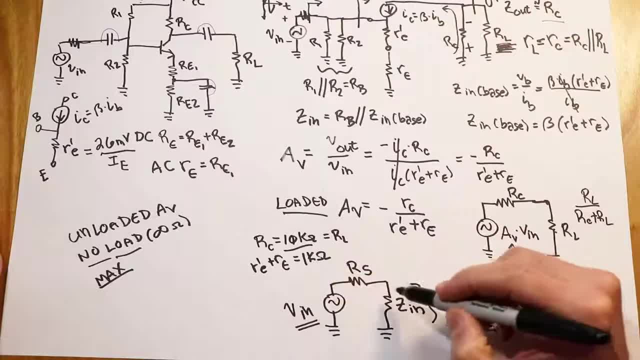 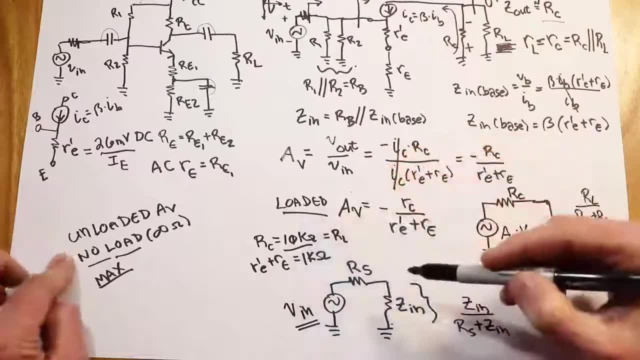 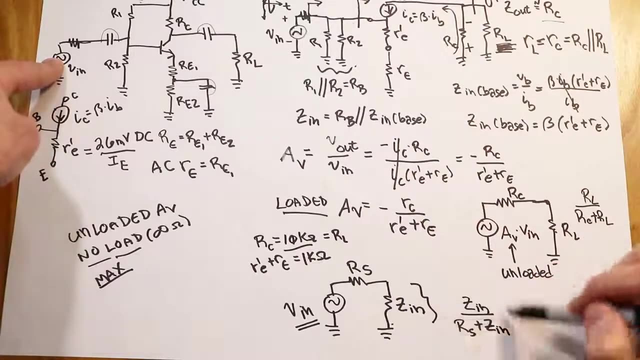 will tell you what that fraction of Vn gets to the input right. So if we calculated the unloaded gain and we have a large source impedance, then we would take our input voltage, we'd multiply it by this little divider here to figure out how much actually gets to the base. 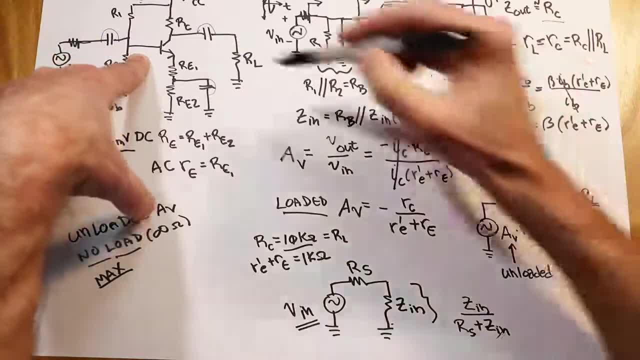 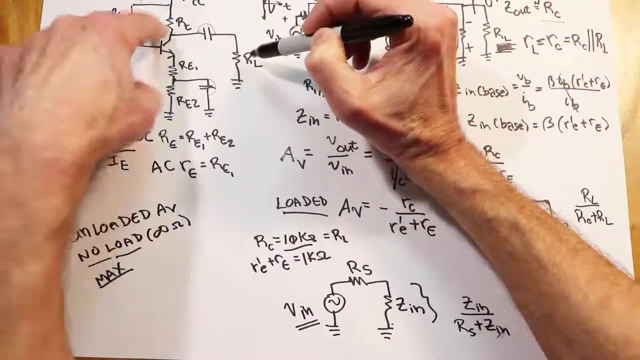 You take that, You multiply it by your unloaded gain, and that would be the biggest possible voltage you could ever get out here if you didn't have an RL. if this was open, right, If we do have an RL- that voltage would then be split down. 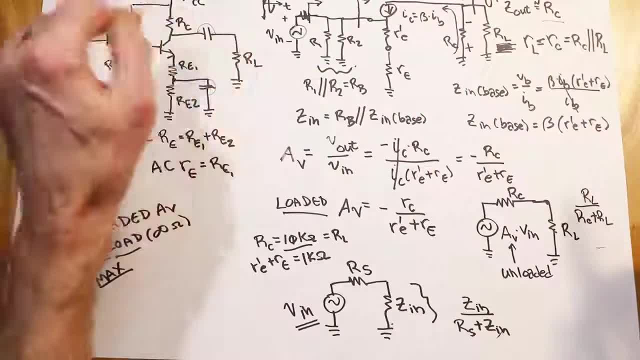 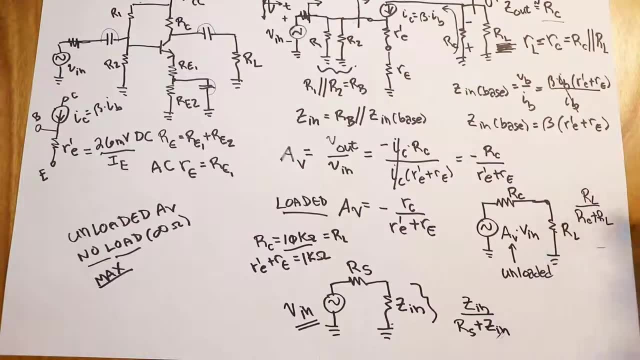 in accordance with this voltage divider right, Or, as I said, if it's fixed, we could just figure out what the loaded gain is and go from there right. So if we come up with a gain of, you know, 100,, 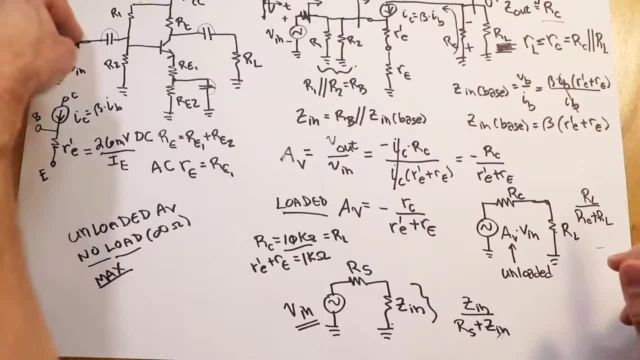 I'm going to have maybe 1 millivolt coming in here. If we can ignore the source impedance, then that 1 millivolt's going to get multiplied by a gain of 100.. We're going to see 100 millivolts out there.